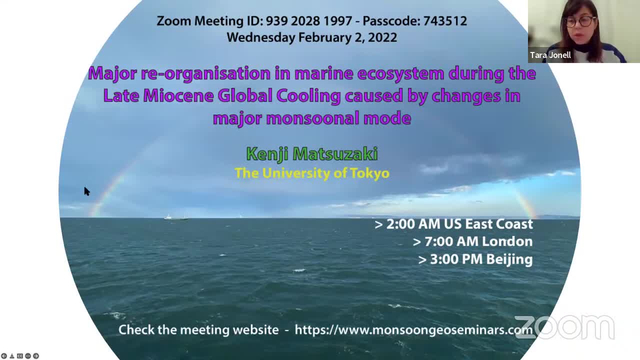 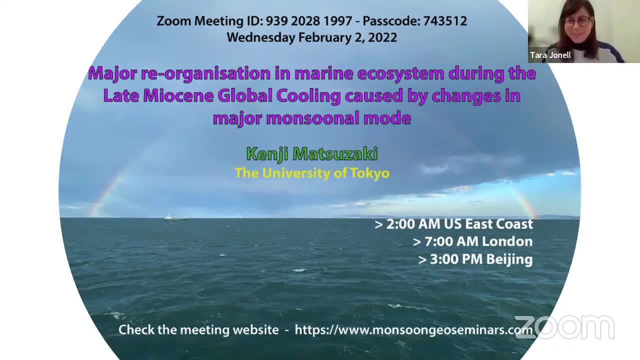 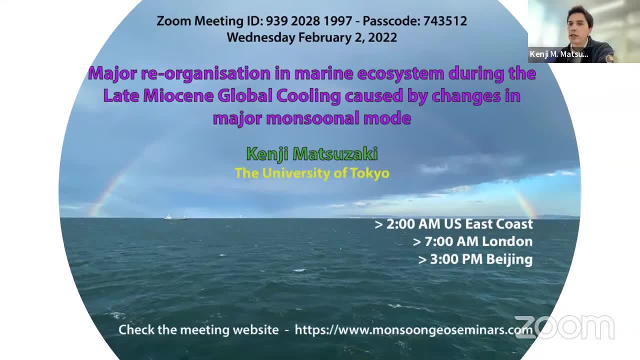 It's almost six years that I'm working with the Miocene sediment of the Japan Sea And I just through this talk, I just try to summarize what I've done during the sixth year. So I focused in this research on the late Miocene. 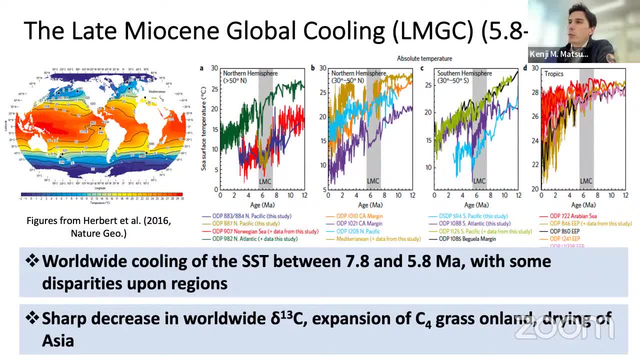 Mars, and because there is a newly very famous global cooling, which is called the late Martian global cooling, which span from 7.8 to 5.8 million years ago, and this event is characterized by a cooling of the mid to high latitude of both hemispheres, as you can see here, in the northern hemisphere and in southern. 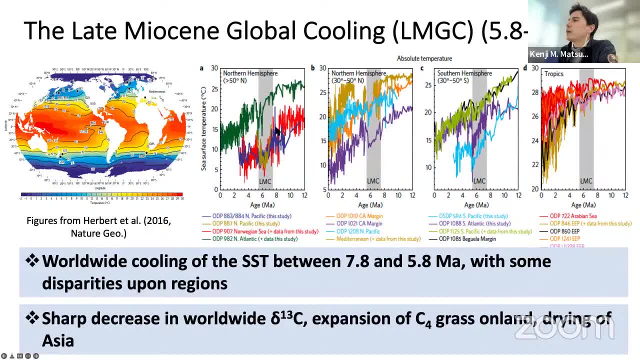 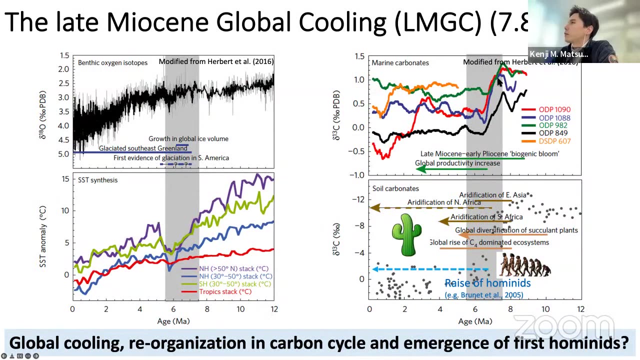 hemisphere you have a sst drop of between 5 to 10 degrees, while in the tropics this cooling is very minor, as you can see, only two to three degree decrease here. but sst decrease is not the unique feature characterizing this cooling event. so this is for compilation of carbon isotope. if, as you can see here, 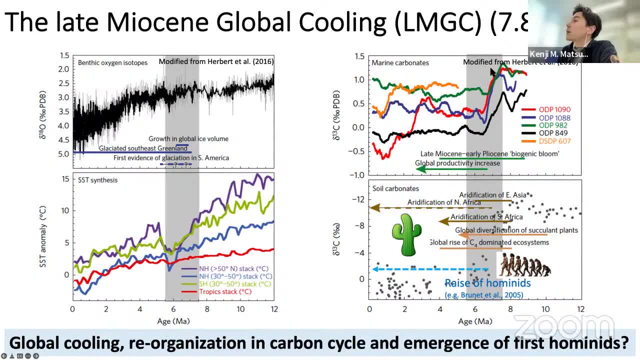 there is also a huge decrease in the global carbon 13 of the deep ocean and many discussion was has done for try to explain this decrease in the carbon pump but that, based on the paper I have read until now, there is no clear consensus. there are 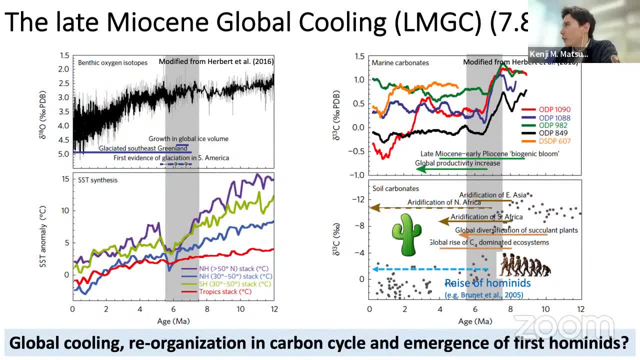 some people arguing for a biogenic bloom. there is also arguing for a change in vegetation, so I think it's not still a reserved issue. however, just when you have this decrease in carbon, it is true that you have a huge vegetation changes in in the world: in Africa and East Asia, where you have the rise of C4 plants and the rise of vegetation. 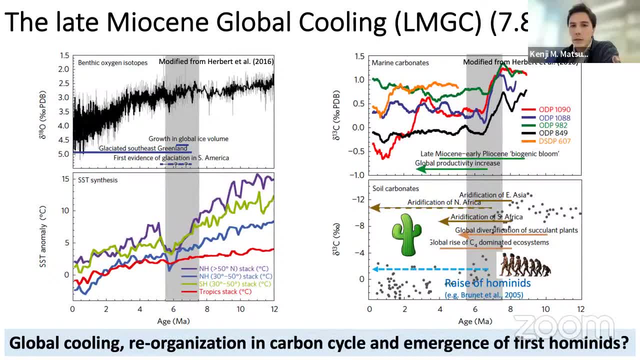 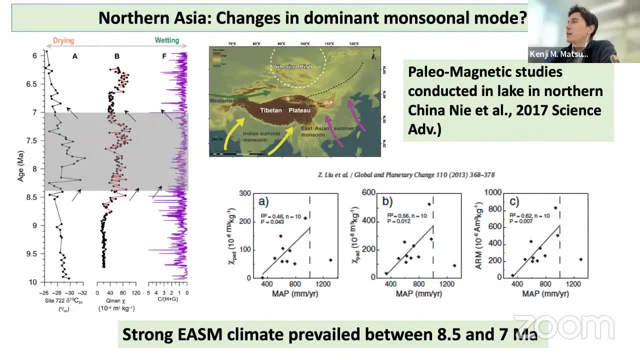 more characterising dry areas, And in Asia, about the climate. there are also many studies which have been done around here, and there are many, so I'll just present the two research I've selected, but it's two among many, So this is a research done in the north China. 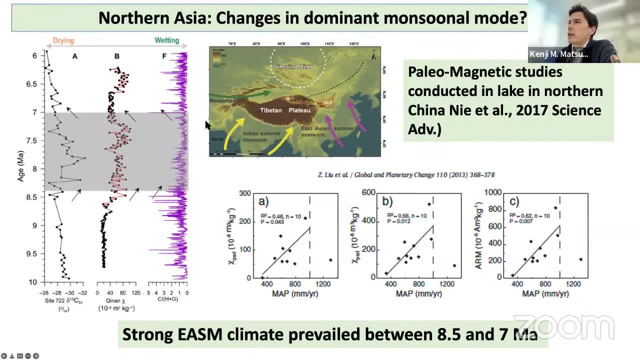 It was conducted in a lake and they did many magnetic susceptibility analysis of the record of the sediment collected from the lakes and because in based on modern calibration, this data fit Of course infer, as you can see here, precipitation. here it's the precipitation year. 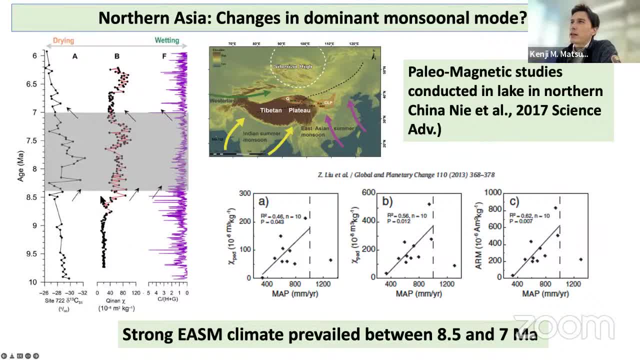 They suggested that between 8.5 to 7 million years you have a relatively wet climate in northern Asia, while since 7 million years it's likely that you have a more drier climate, and they proposed the weakening of the summer monsoon here. 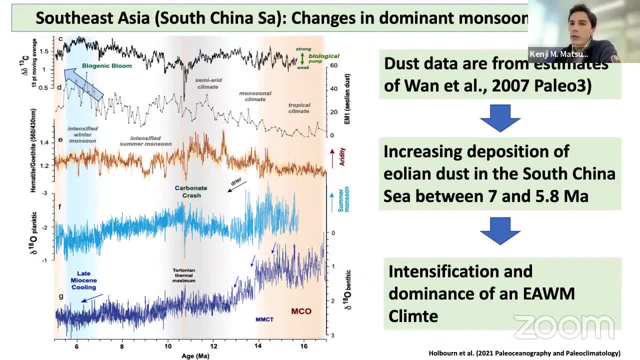 And now I will show some East Ocean data. it's from the South East Asia in the South China Sea. It's a compilation of many data such as oxygen isotope. you have hematode-goetate ratio and Eolian dust coming from a previous study, which is based on estimation, but here also there. 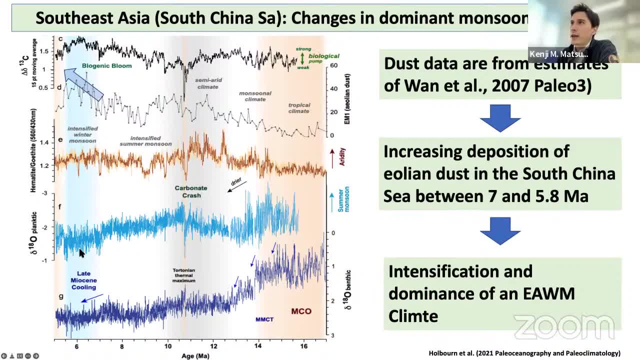 is some evidence showing that from 7 million years there is an increase in deposition rate in Eolian dust, And it's also in the last three months, and it's also not confirmed that the winter monsoon get intensified at that time, Which is in agreement with the weakening of the summer monsoon in North Asia. 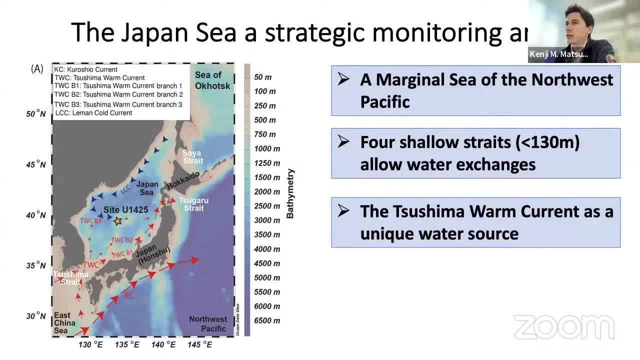 So the first step, what I wanted to do here, is to try to monitor such changes in the monsoon, but in the Japan Sea, Because the Japan Sea is a very particular area of the Japanese oceanography now. but the most important thing is that it's highly influenced. 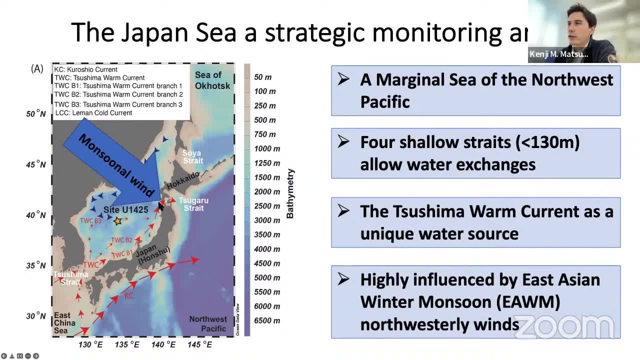 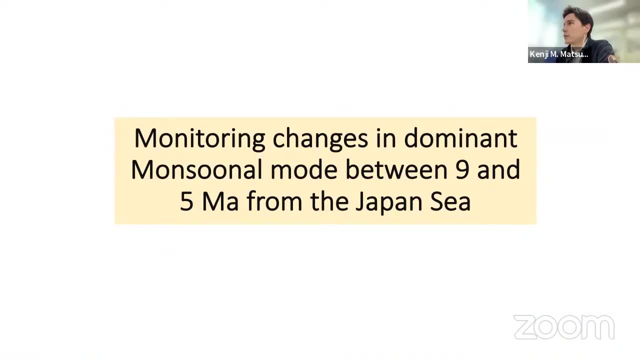 by the monsoon. So by doing an analysis over there we thought that it is possible to reconstruct monsoon variability during the Miocene. So this is what we target in the first stage. So first we try to monitor the dominant monsoonal change between the Miocene in particular. 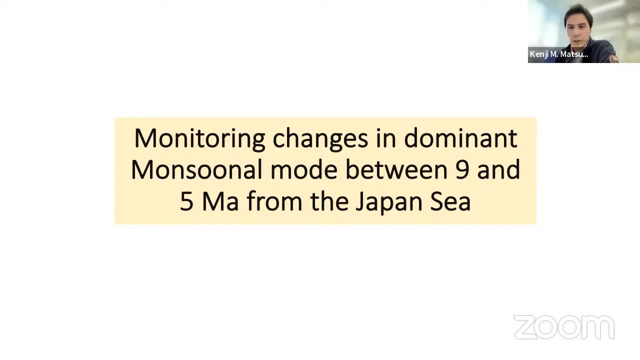 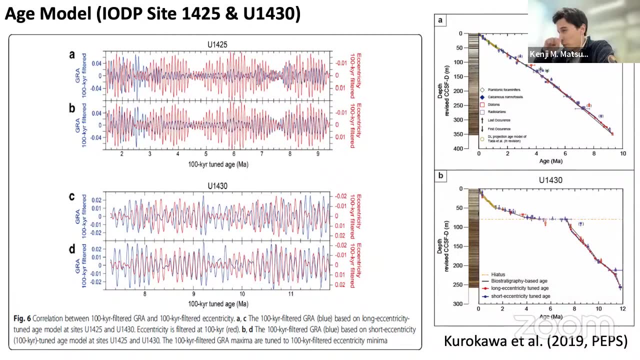 between 9 and 5 million years in the Japan Sea, And for that we need an accurate depth-age model. So this is the first step. Primarily, we did the biocertigraphy depth-age model and based on this biocertigraphy depth-age model, there was a tuning of the sediment. 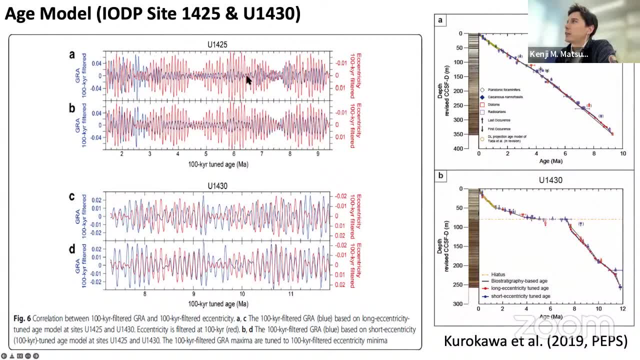 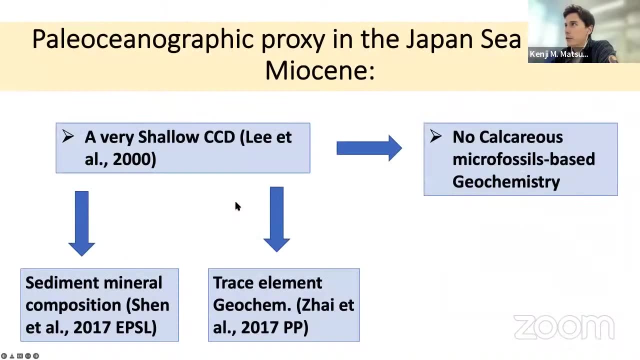 gamma reattenuation rate to the Milankovitch cycle to try to get the most accurate position. So this is the possible depth-age model for trying to constrain well the monsoon variability during the Miocene. And the next step, what you need is proxies. But in the Japan Sea there are a few problems. 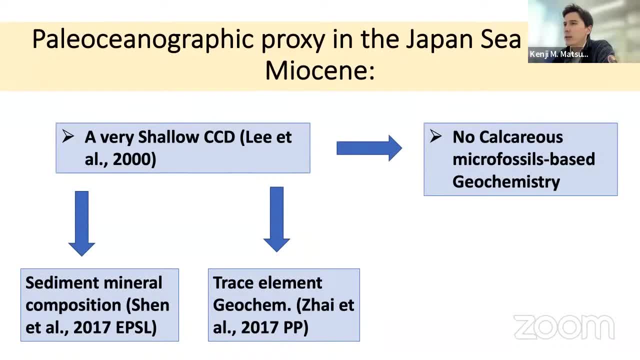 because the CCD is very shallow, so there are not many calcareous microfossils. so all calcareous microfossils by geochemistry is not very likely possible here. So most people try to do something with sediment, mineral composition, Also trace elements, geochemistry And mainly 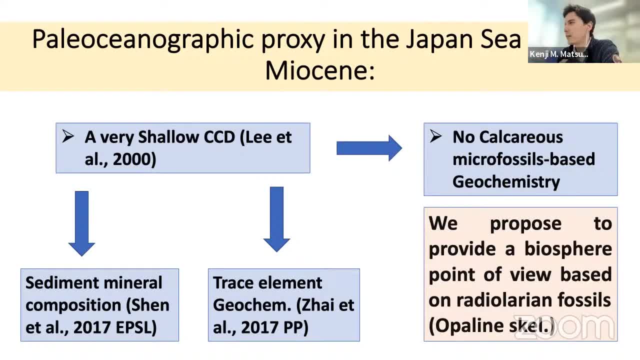 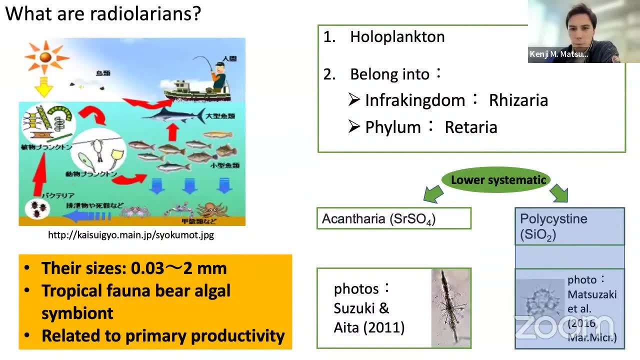 because I'm a microp turbulentologist, I propose a new semiquantitative approach for trying to reconstruct the monsoon. I propose to analyze Raduarion microfossils because they're very well preserved in such sediment. I don't know if you are very familiar with Raduarion, but they are micro fossiles, so metropolitan structures. What it would mean is that they would have a сопир wilderness and the salmon, the fish and the fish itself would also be uncomfortable. And of course, products of chemical industrial, such as sigel, require less popularity and do not perform. 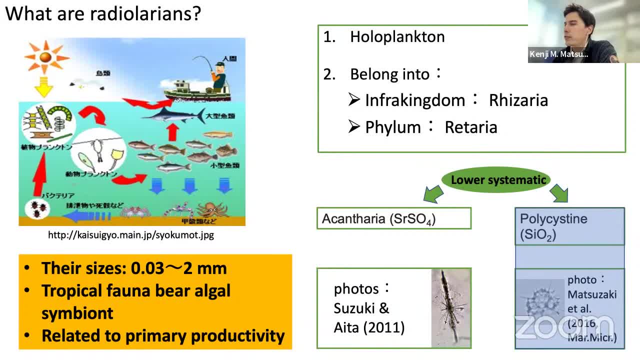 well during the 37th of July period, and less dirt and the sediment and the deposits on the L Tschuk holoplankton, their size from 0.03 to 2 mm, and some tropical fauna, bear, argar symbionts. 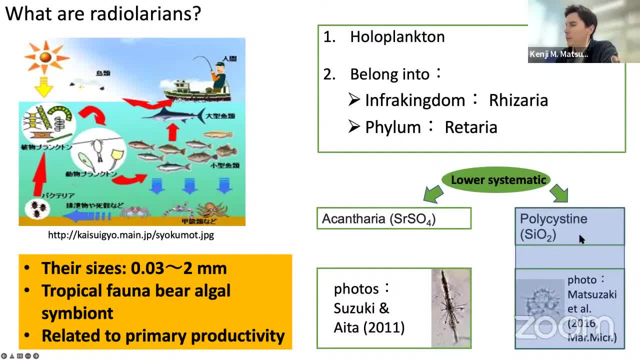 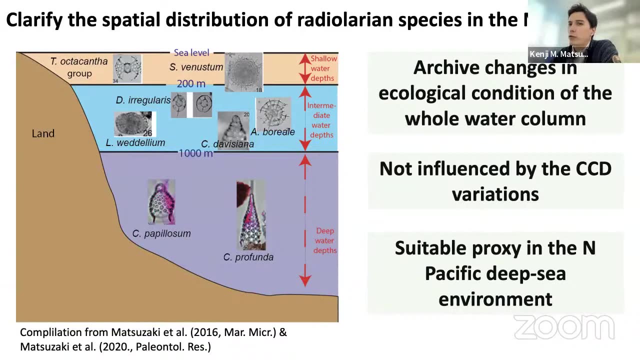 and they bear a skeleton based on biogenic opal, so they also have the potential to be used for discuss variation in the silica cycle. So what I've done for my first research was to try to develop this microfossil as a pyrocynographic proxy in the North Pacific. 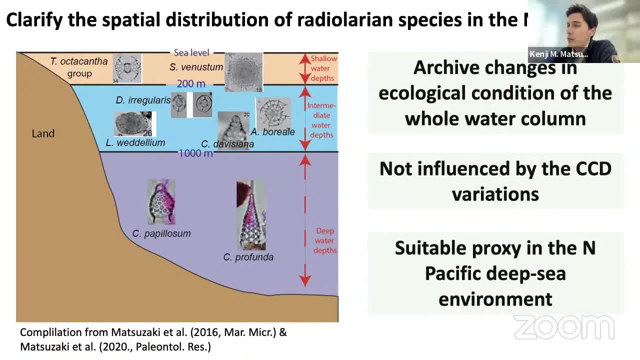 So, via many offshore expeditions in the North Pacific, I analyzed plankton samples from the surface of the deep water and I get to the conclusion that this is more likely the vertical distribution of Rhodauralia in the North Pacific. So it's very well stratified. 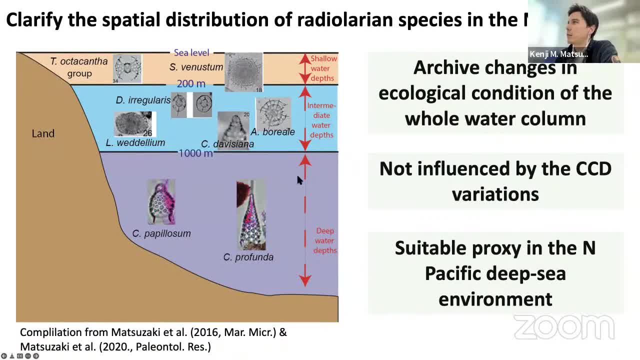 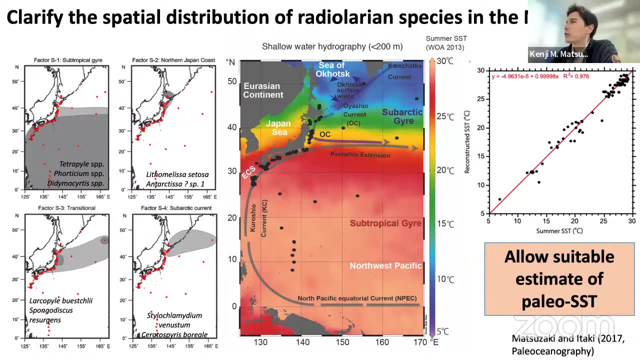 You have surface intermediate and deep water species, so it can be very useful for reconstruct shallow to deep water marine environment, in particular in area where you do not have carbonate. Then we also need to know where species live, so as a first step I try to qualify their 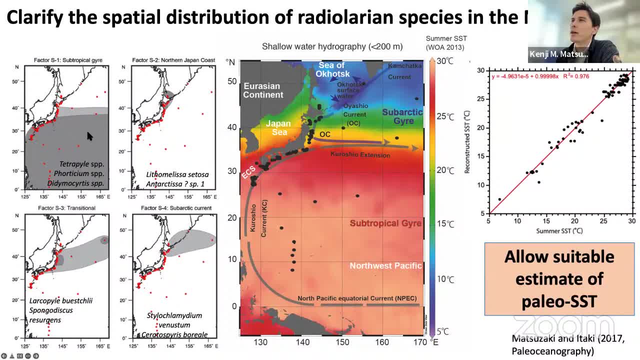 biogeographic distribution. This is what I've done here with this group here. so the conclusion is that you have species who live in the subtropical area, the transitional area, the sabbatical area, so it can be used for pyrocynographic studies. 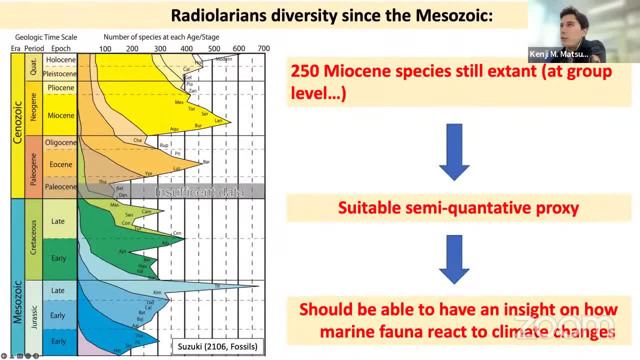 And for the mouse. but when you deal with very old sediment, the problem is that you do not know. you do not have many information about where the species live and about their ecology. But the good point, as you can see with this graph figure, I'm pretty sure it's a good point. 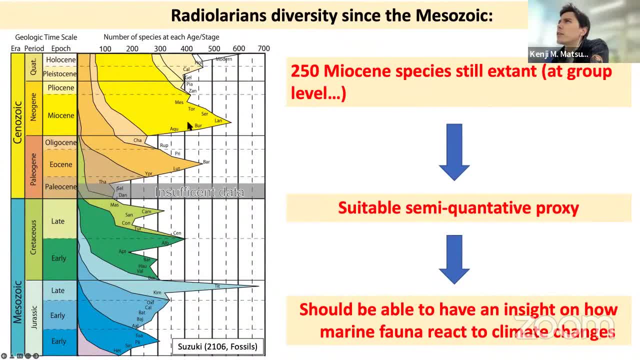 So the problem is that you don't know where the species live and about their ecology, but the good point, as you can see with this graph figure, I'm pretty sure that you have a good point. This figure is showing the number of species since the Mesozoic and the miocene is here. 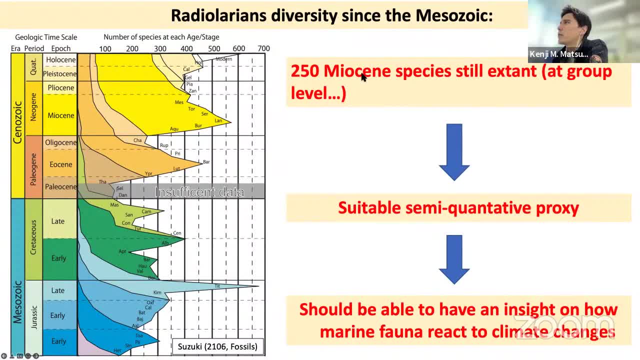 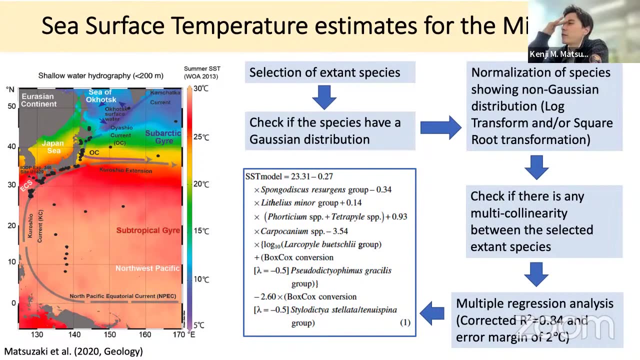 and as a summary, you have almost 250 miocene species still extinct. so we probably know their ecology. so pyrocynographic studies of the miocene basin should be possible. The first step. what I wanted to do in the Japanese sea is to know how the sea surface. 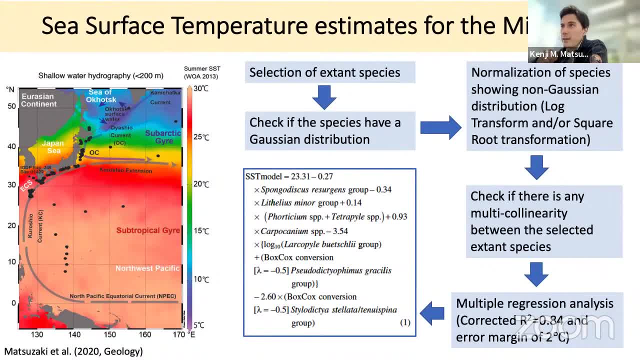 temperature have changed. Under temperatures she's much more active than Bermuda after being exposed to the sea at that time and because no forum, I tell before. so magnesium calcium not very possible. so I try to apply a transfer kind of multiple regression analysis for try to get sea surface temperature for the medicine, only relying on extant. 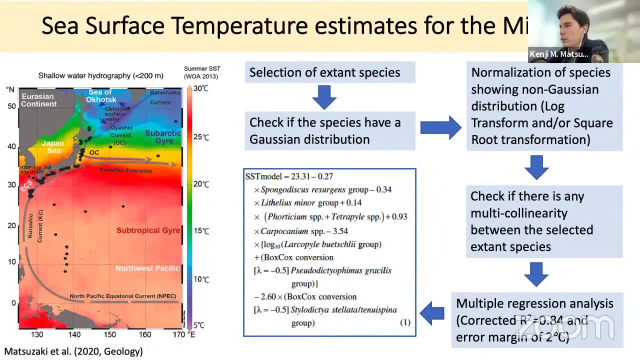 species. but the problem is that because there is no, there is no high diversity in the species in the Japan Sea so we had only eight extant species groups. so we did some statistic for try to get quite suitable equation for discuss changes in sea surface temperature in the marathon. but even if we can have 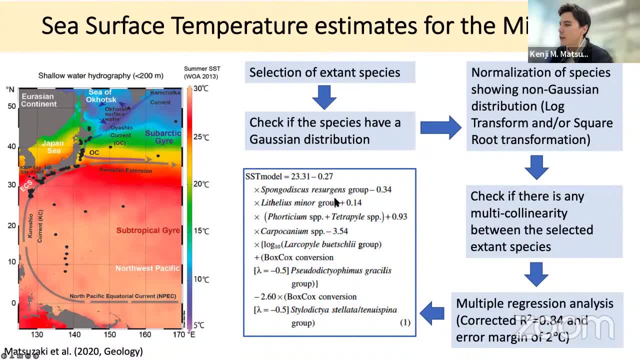 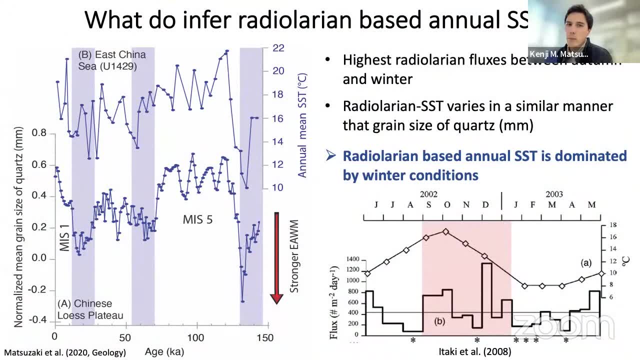 temperature based using this equation. we have to know what this temperature mean. so for that we did, we first proposed to apply it on quaternary, on for the quaternary. and this is the figure you have on the left. so in the left part above you have the sea surface temperature steam obtained. 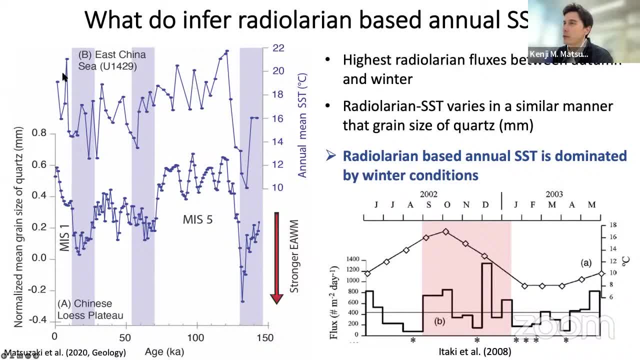 from the equation I've shown. I show you above using radialian. this is a. it is. it is also an IODP core, but collected in East China Sea for the Pleistocene. and here you have the, the normalize main great mean grain size if obtained from the Chinese last plateau. 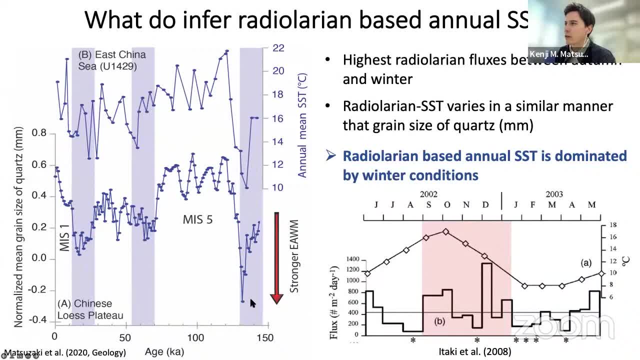 and here you have the age and, as you can see here the blue band indicate glacial period. so during glacial period is the. for the quaternary, using the method above, you have very low sea surface temperature which correspond to period of strong winter monsoon. so it is likely that, based on the 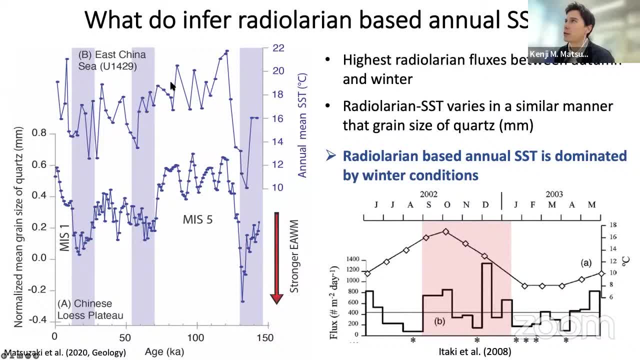 this method for the quaternary, you can reconstruct sea surface temperature, which fluctuate according to the glacial interglacial cycles, and low SST seem to seems to be related to strong winter monsoon and for further support that hypothesis, we propose to examine to discuss the seasonality of radialian in. 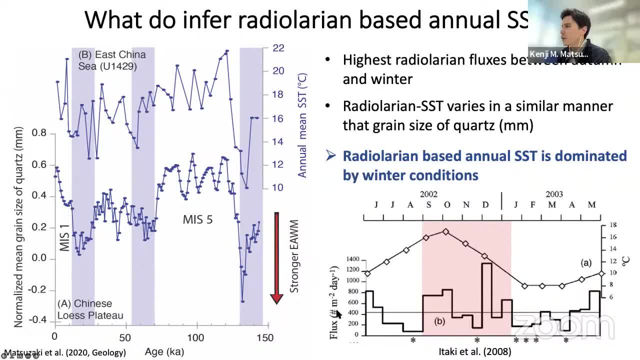 the Northwest Pacific. so this is the flux of the speed, the daily flux of radialian species in northern Japan, and there is one that, as you can, there is very few peaks, but the highest peak is reached in December, so it's, it is likely that radialian is more. 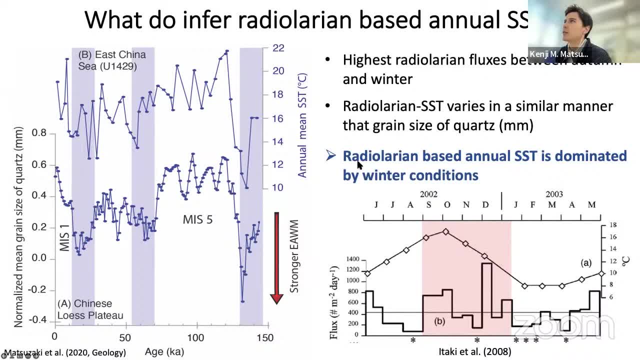 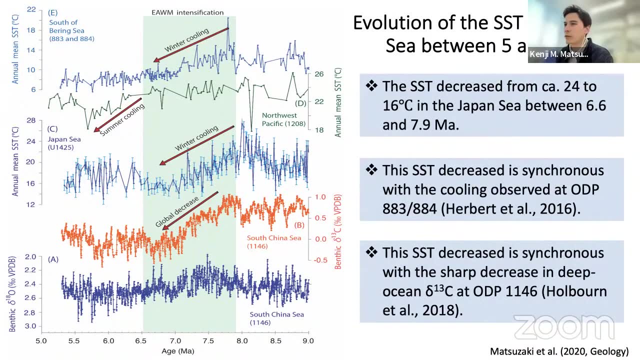 likely in frame condition during winter. so we associate the radialian temperature to winter SST and thus it fit well with what we have on the left, which is strongly related with the winter monsoon. so all the preliminary done, now we propose to reconstruct the sea surface temperature of the massing in the Japan Sea, the 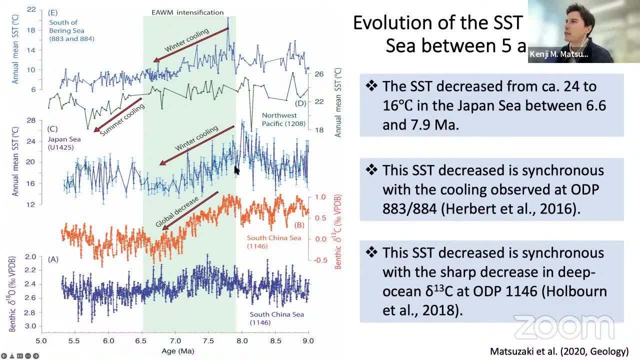 Sea, Japan Sea. this SST profile is what we get from radialian, and we then compare it with Benzic carbon profile and oxygen isotope profile obtained from the South China Sea, and above you have Arcanine SST obtained from the south of the Bering Sea and the Northwest Pacific. it is a Schatzky. 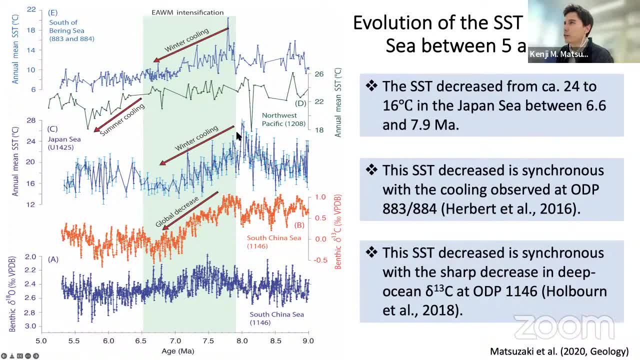 So the key point was that we have a strong cooling in gradual necessity from 7.9 to 6.5 million years, where the temperature decreased from 24 to 16. And this cooling is very synchronous to what you have in the carbon-proven South China. 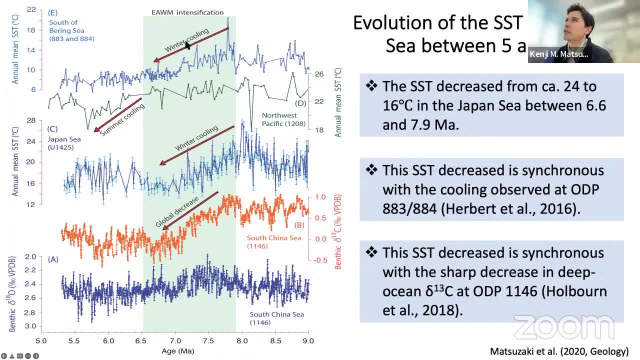 Sea And this is also very similar to the cooling observed in the Bering Sea. So if you just look at the radial hand curve and based on the assumption we did previously, it will infer that we have a cooling in the winter SST due to a strong East Asian winter. 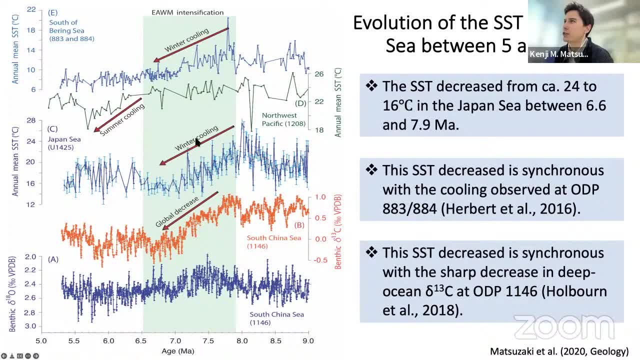 monsoon between 7.9 to 6.5 ma in the Japan Sea. But if you looked, for example, here at Schatzky- Same latitude- You do not have the cooling. It's much lighter. So for trying to discuss this disparity, we just check when you have the maximum bloom. 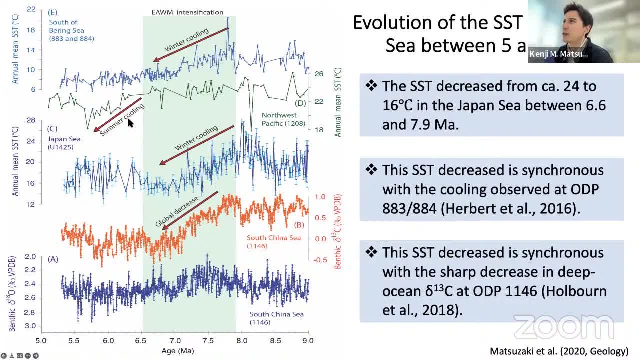 of alkanon of nanos in the Northwest Pacific. It seems that alkanon bloom are higher in spring to summer. So this discrepancy may be related to disparity in the season. The summer cooling may happen later and the first you have and the late-margin global cooling is first characterized. 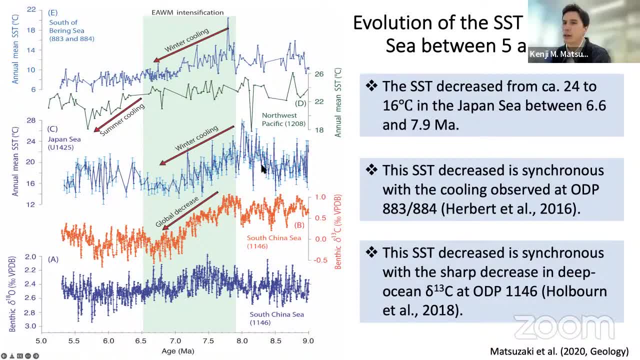 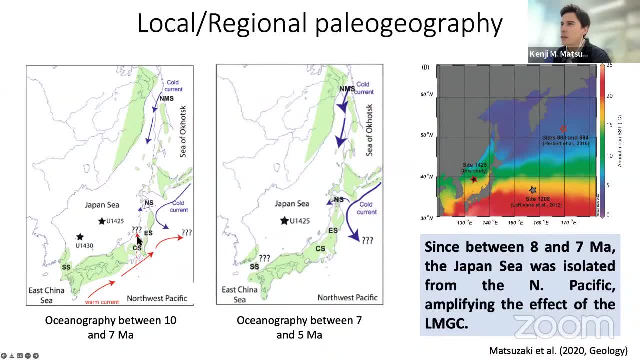 by a strong winter cooling. This is the hypothesis we get in the first step. But also the Japan Sea is also characterized by tectonics and about 7 million years it is likely that you have a very shallow seaway here which allowed inflow of warm water. 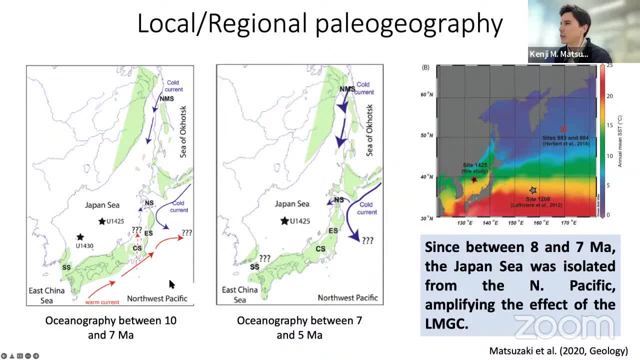 and this seaway likely closed around 7 million years. So this is a very good hypothesis, Thank you, So it is. also We suggest that this The closure of the deep seaway around 7.. Between 7 and 8 million, highly amplified the cooling observed in the Japan Sea and 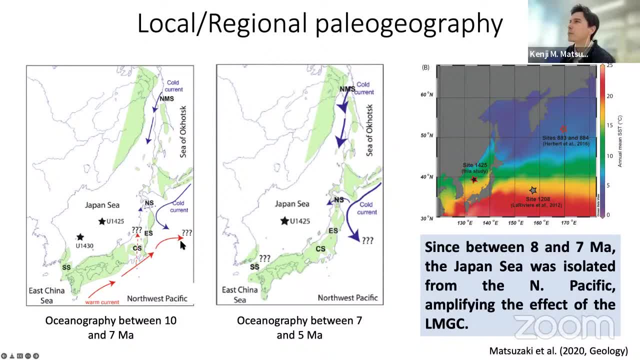 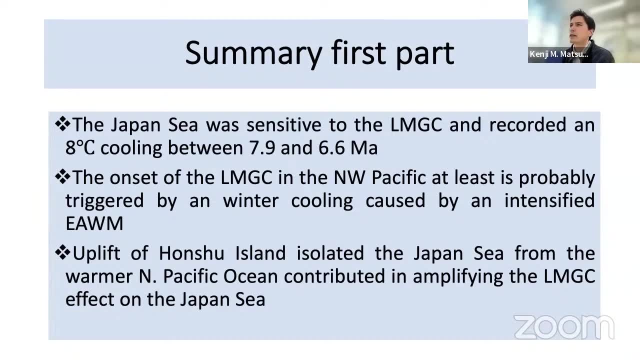 also may contribute to the drastic cooling we recorded above. So here it is the summary of the first part, where we show that the Japan Sea recorded an 8-degree cooling between 7.9 and 6.6 million years, and this cooling was probably amplified. 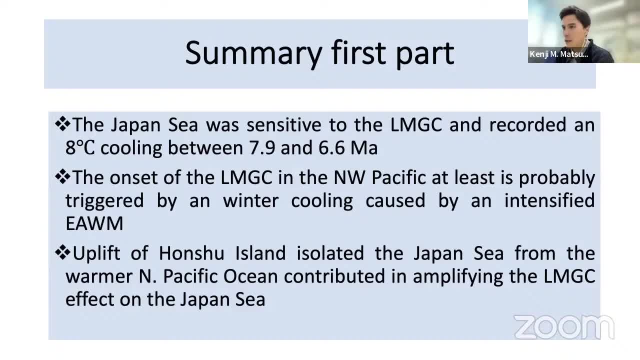 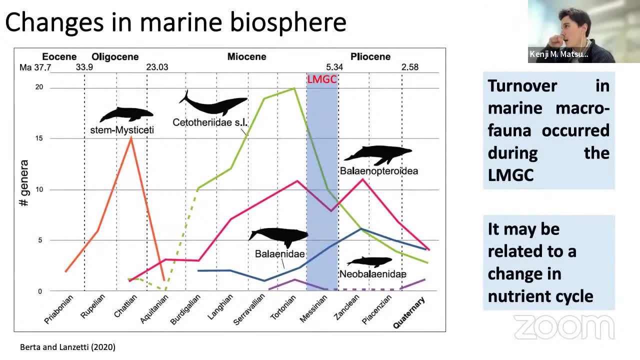 by tectonics. Now, in the second part, I wish to focus on the changes we had in marine biosphere, because during the LMGC, which is about here, you have many turnovers in macro-fossil macro-fauna. 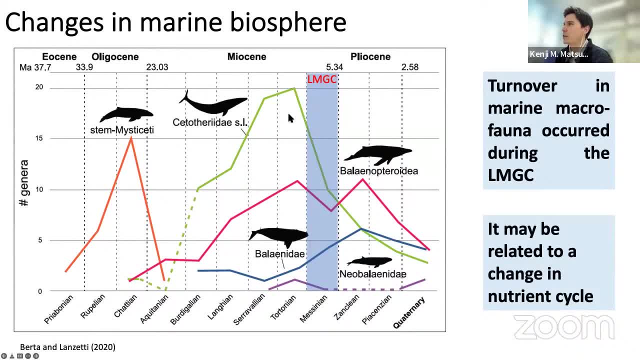 and here I show. this is the case of the Balinidae, as you can see here, with the decrease of the ancient type of whales instead of the more recent type of whales. But this is just one example among others. There are also many other marine mammals who evolved or changed. 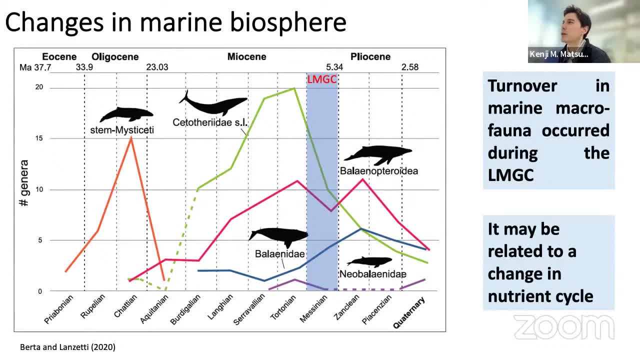 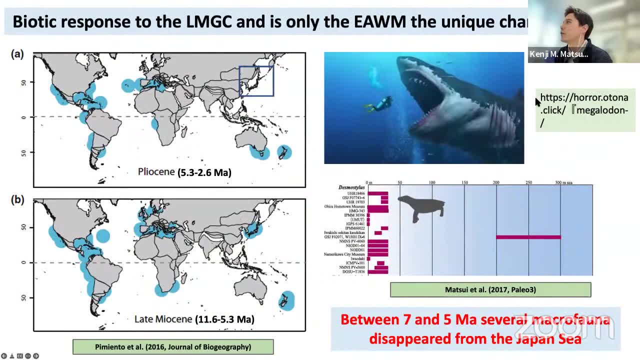 at that time. so it is likely that there is a drastic change in the marine mammals during the lead marmots in global cooling. And if you get another focus, this is for the shark, a megalodon, as you can see here. This is the distribution of these sharks and this 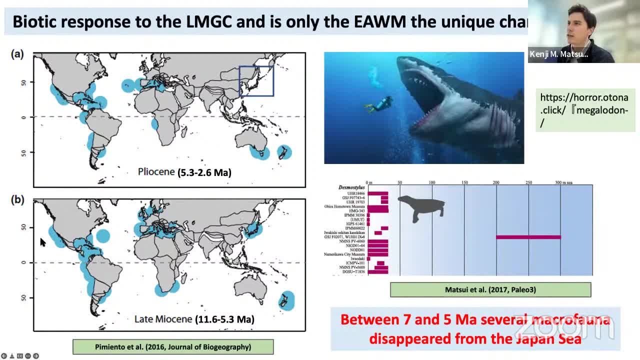 shark until 5 million years and its distribution between 5 to 2 million years. and you can see the Japan Sea is here and it is likely that during the late Martian global cooling, this shark stopped to inhabit the Japan Sea And at the same time, you have another mammals. 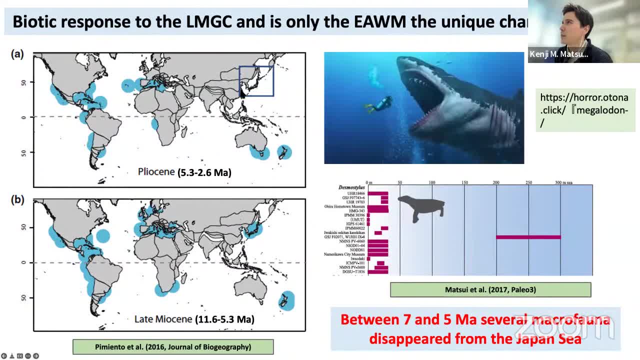 who inhabited the Japan Sea coast, who disappeared during this time interval. so yes, during the LMGC you get a drastic macro faunal turnover here and changes in the monsoon mode. as previously, we showed that we get a dominance of the winter monsoons in the LMGC, so it is possible that 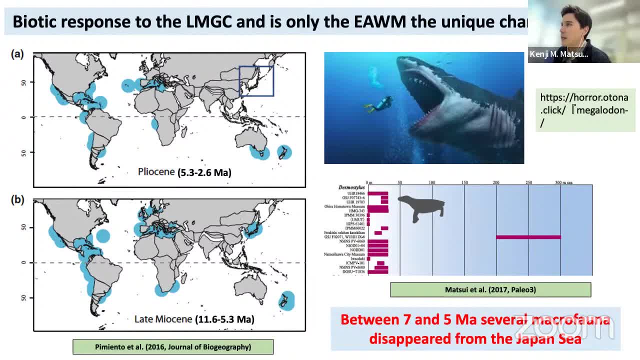 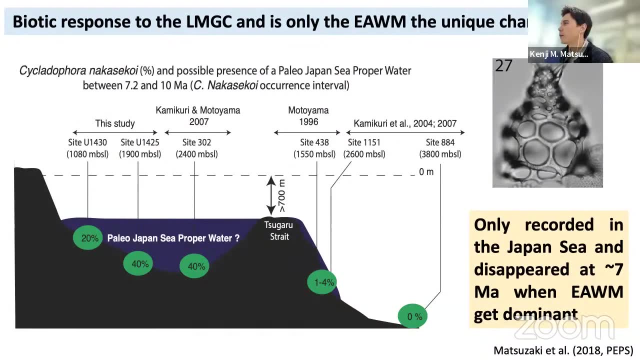 the cooling and the drying of East Asia may cause this great faunal turnover, but we will probably have to wait and see. We propose to discuss it a bit more in detail because if you look, for example, at the Radular and Fauna, you have an endemic species, this one. the name is like this, but this species 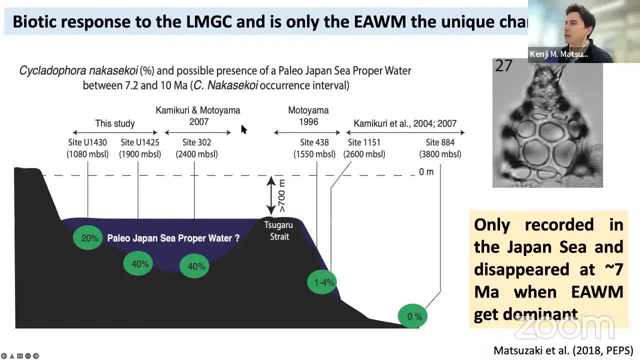 only inhabits the Japan Sea between 10 to 7 million years and it disappeared during the LMGC. and because it is endemic to the Japan Sea, we proposed before that it may inhabit deep water of the Japan Sea. It was isolated with the North Pacific because you have a stretch here about 1,700 to 1,000. 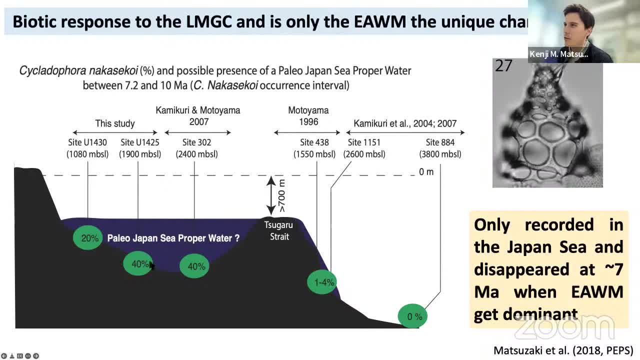 meters, which isolates this species geographically. But if it's really the case, if you just have, if it's really the case, monsoonal change may not likely affect deep water. So deep water, you know, it's more related, it's more surface processes. 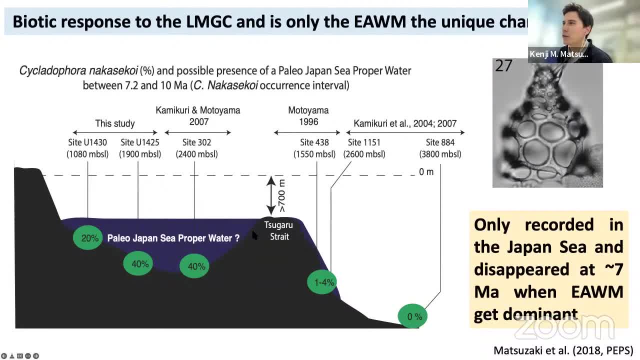 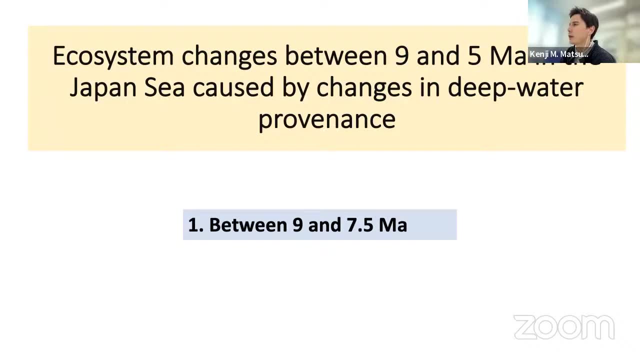 So we suggest it is possible that there is a kind of change in deep water exchange or circulation of the Japan Sea at that time as well. So this is what we propose to qualify here. And, yeah, so we propose to qualify deep water provenance of the Japan Sea between 9 to 7.5. 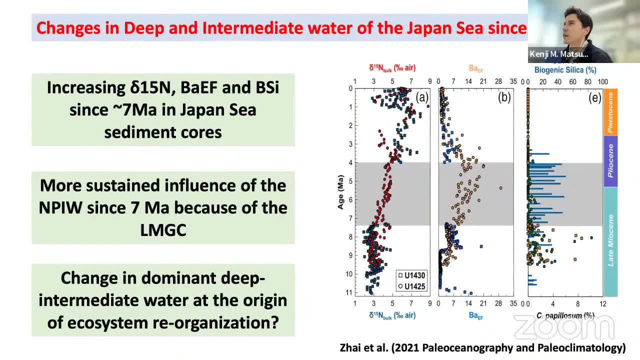 million years. It was already reported that during the LMGC the NPIW get intensified and likely influence the bottom water of the Japan Sea. So, for example, deep water endemic to the Japan Sea will okon Me. so that means for 30 years where it's more Abbott and wets weather than 2000 years. 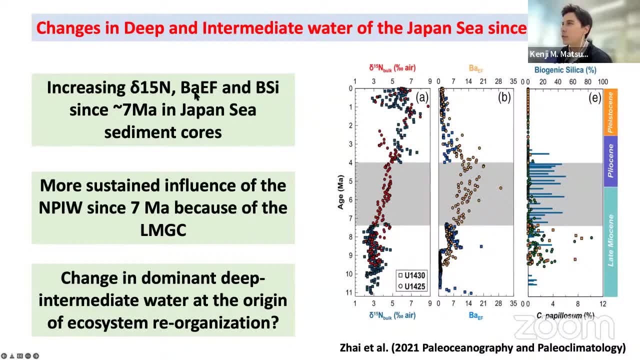 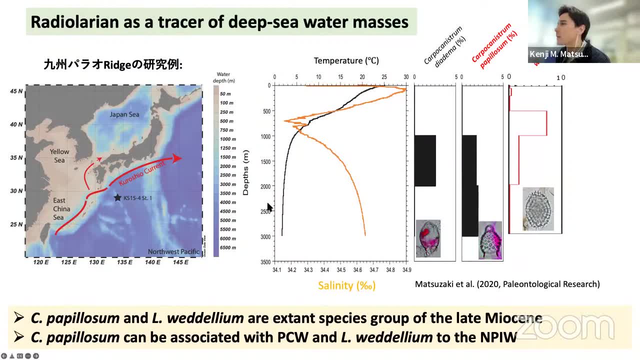 So naturally deep, really offer a greater level of flexibility in the flowering layer and the fim of the material, And so from that we've humour the axes in in the bottom water because we- just you- stepped under the bottom. програмing, working, Post-working, more background environment. 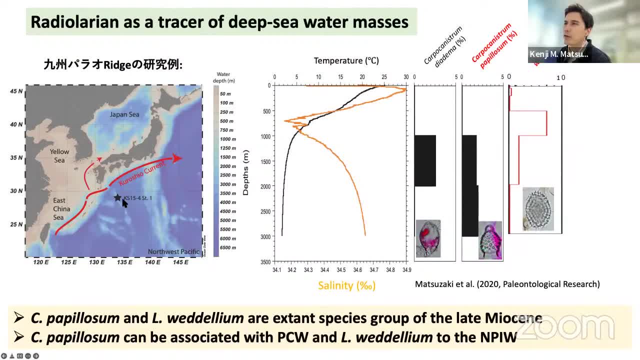 Prof González- Yeah, yes, exactly, Prof González- And we made a direct connection from the Jan. Second fundamental questions I collected here of the Northwest Pacific. We get plankton towers from 0 to 3,000. 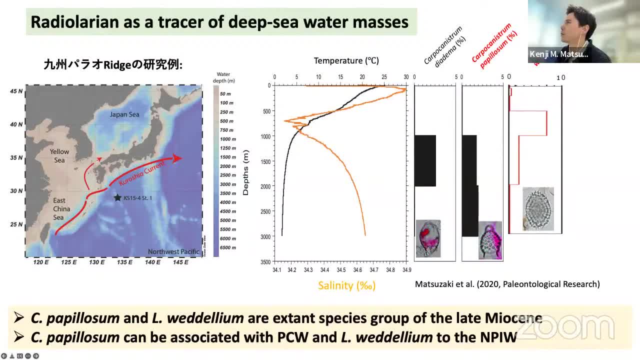 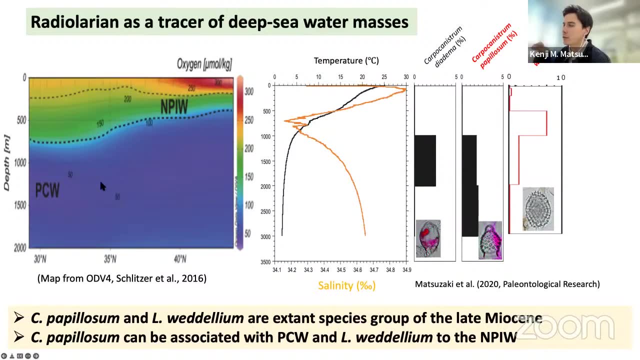 meters and we want to focus on these species, in particular those in red, because this is the two extant pieces occurring in the miles in sediment of the Japan Sea And this is the profile of this oxygen profile of this area, of the point I've shown you just before. So here, from 1,000 to 3,000 meters, 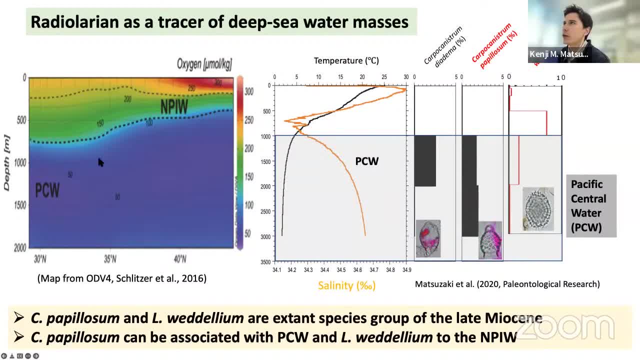 which corresponds to water depth very with low oxygen, distilled oxygen, and we associate this water mass with the Pacific central matter, which is originated from the Southern Ocean, which is very nutrient rich but poorly oxygenated and quite salty. And at this water depth this radial area is abundant, While above, for example, 500 to 1,000. 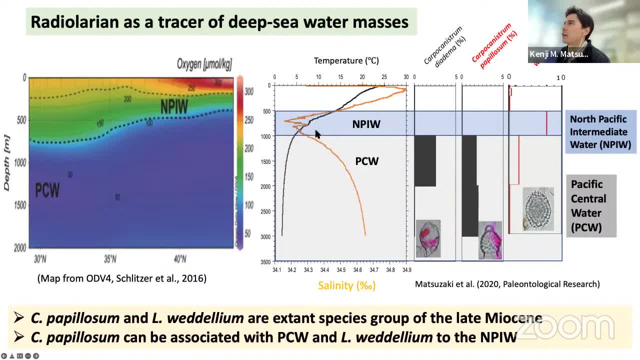 meters, which is more oxygenated and, as you can see here, the salinity is very low saline and very low temperature water. you have these species, which is very abundant, and this water mass actually corresponds to the North Pacific intermediate water. So now we propose to discuss change in the accumulation rate. 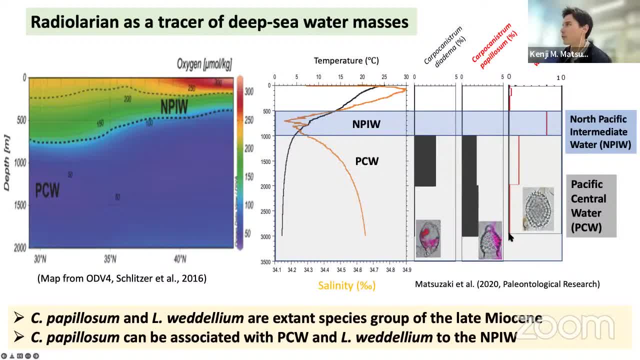 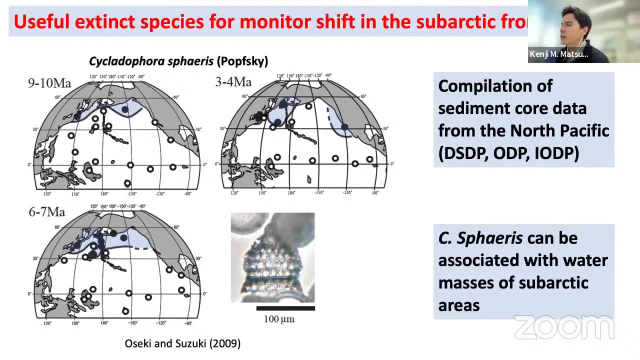 of these two species for try to discuss the deepwater provenance of the Japan Sea. at that time We will also use another species for try to relate it with the changes in the surface, which is this species, which is an extinct species but, as you can see here, 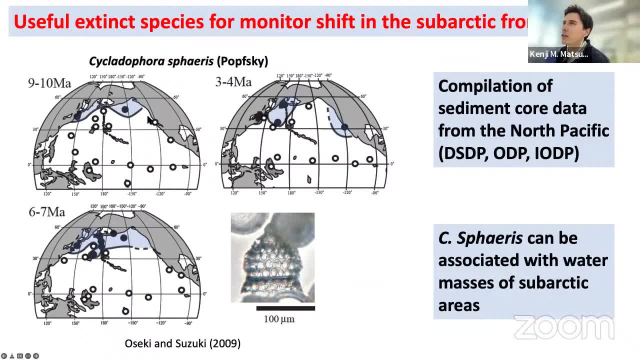 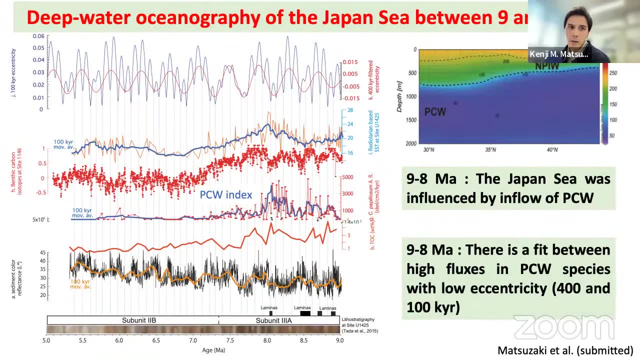 before the lead-maiosing global cooling is restricted to the very high latitude and with the lead-maiosing global cooling it shifts until the mid latitude. So this species can be used for monitoring the southward shift of the subarctic front. So now I will show you the main data, So I will propose to. 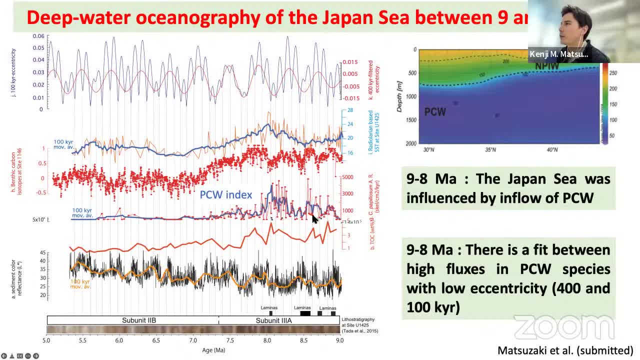 focus on this curve, the PCW index. This is the species I've just shown you before, which is related to the Pacific Central Water, So its accumulation rate varies from 0 to 5,000, and high abundance of these species as 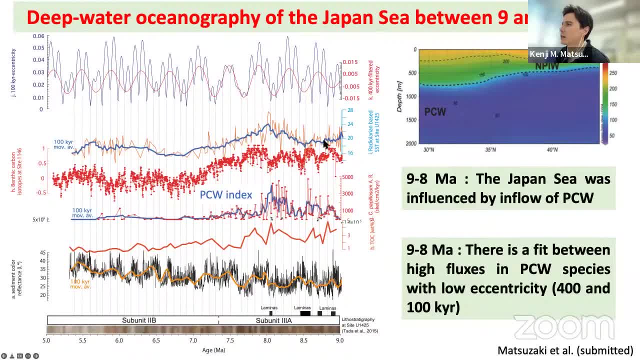 you can see here most likely occur when the eccentricity is low. So it is based on this rough figure. we can say that it is likely that the Japan Sea is influenced by very deep Pacific Central water from 9 to almost 8 million years and its inflows are regulated by the. 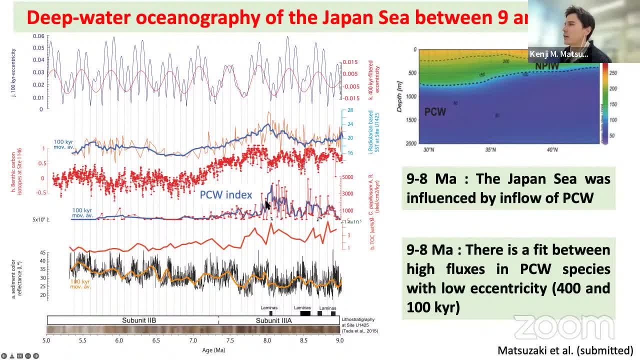 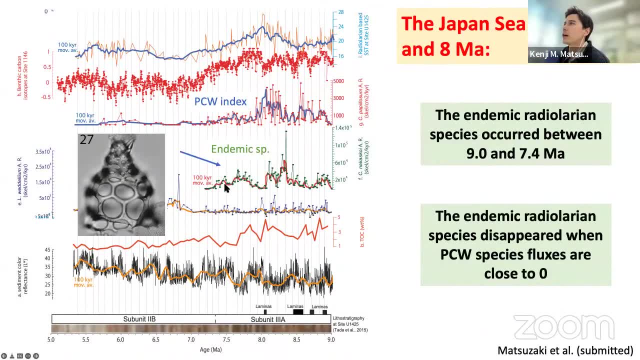 eccentricity and it is likely that you have higher influx of these species during when the eccentricity is low, And here I've plotted down the endemic species I've just told you before in green. and the endemic species occur, interestingly, just when you have. 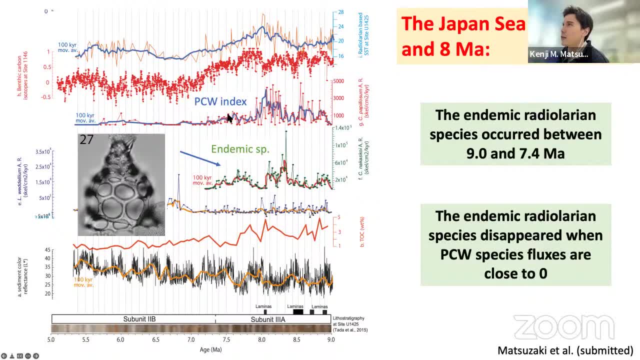 inflow of Pacific central water into the Japan Sea And its high flux also is likely based by a kind of eccentricity and more likely occur when the eccentricity was low. So based on this we can think that the endemic fauna occurrence in the Japan Sea was. 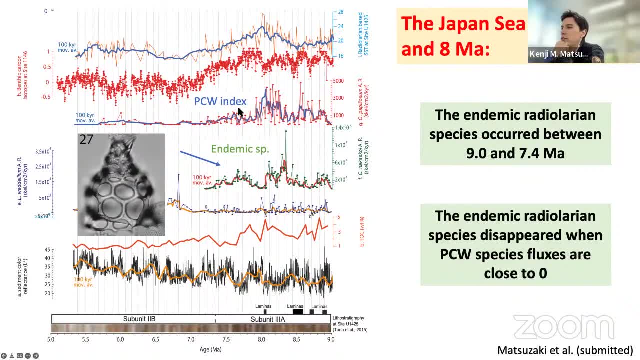 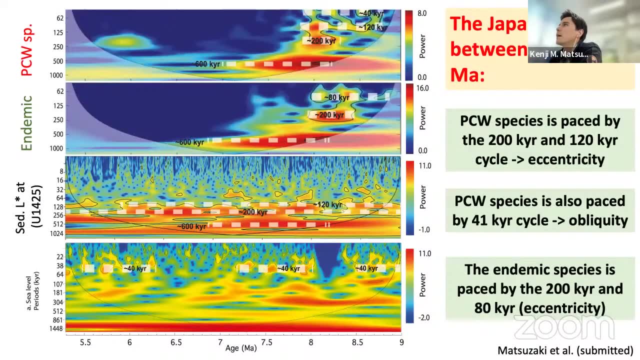 likely related to the inflow of the Pacific central water, at least until extinction, at around 7.4 million years. This figure is not so important. we just showed the main Milankovitch cycle influencing the inflow of the PCW which, as you can see here you have the 200,. 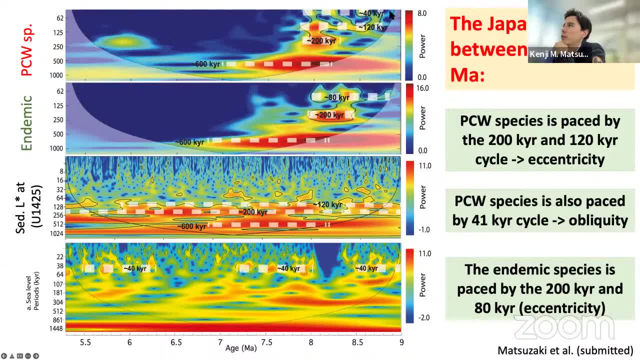 120 and the 40 kilo year cycle here. So these two cycles are the classic obliquity and eccentricity cycle and the 200 cycle is a bit more particular, but in recent paper it was associated to a particular eccentricity cycle. 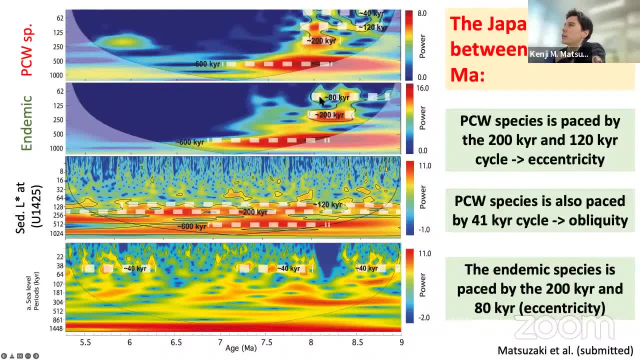 In the endemic fauna we do not have the obliquity but we have a kind of eccentricity cycle which is quite prominent from 8.9 to 8 million years. So in the slide before we saw that we have inflow of Pacific central water during. 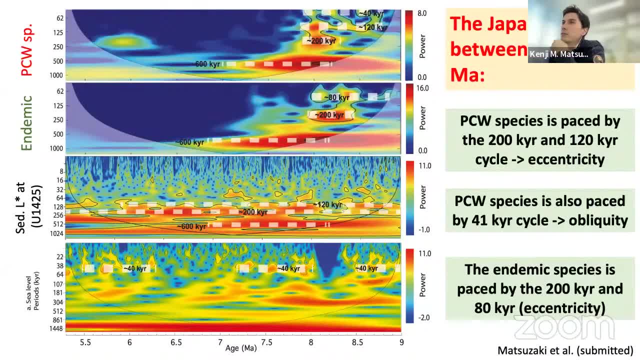 low eccentricity interval, and this inflow is likely necessary for the endemic species to bloom in the Japan Sea. So now we just propose to discuss what is the mechanism which causes the PCW inflow into the Japan Sea and why it occurs mainly when the eccentricity is low. 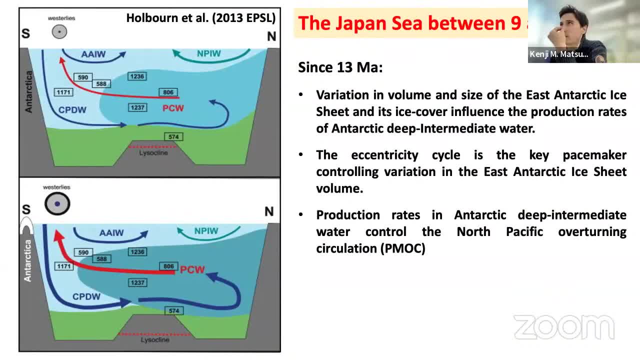 So for that I will mainly rely on Horbun et al 2013 EPSL paper, and it was suggested that during low eccentricity interval, this is the lower part of the figure. here you have an expanded ice volume, an expanded ice cover. 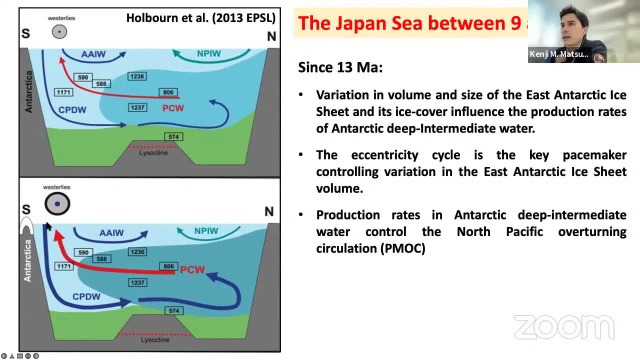 and this will create an enhanced ventilation of the regional intermediate and deep water, which will in turn strengthen the Pacific meridional oscillation and thus we will have a more intense production rate of PCW water, And this occurs during low eccentricity. 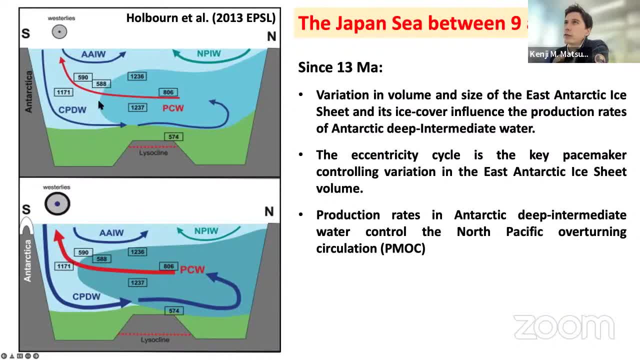 Why The eccentricity is high? because it's warmer, you have less ice. dry sheet is smaller, you have less ice cover. so the Pacific meridional overtoning circulation is lower and thus lower PCW production rate. So this idea is very interesting because it quite fit well. 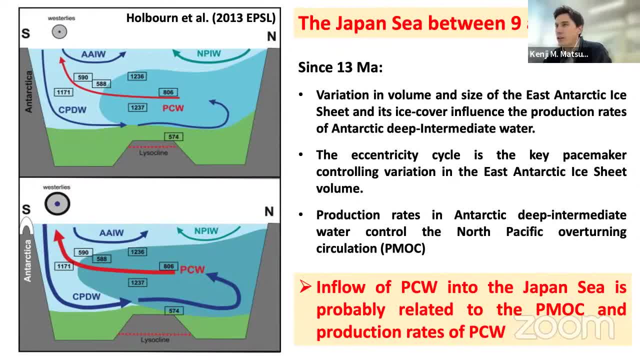 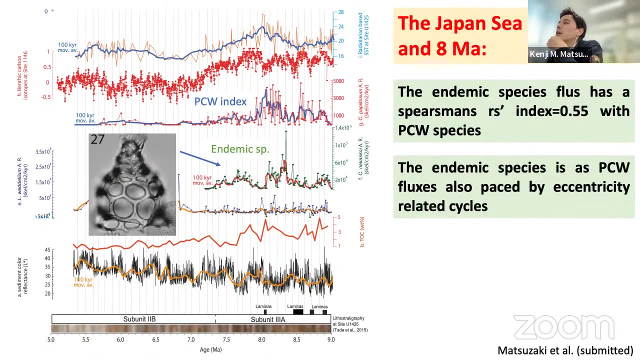 with our record and it will suggest that you have Pacific central water inflow into the Japan Sea during low eccentricity because of an expanded East Antarctic ice sheet and its related ice cover. So we have explained this curve. so this curve just means that you have influence. 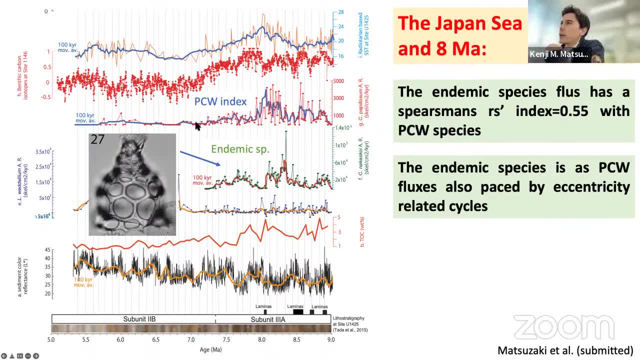 of Pacific central water when the Antarctic ice sheet is quite big, which will strengthen the Pacific meridional overtoning circulation And this will in part allow the blooming of an endemic species. but this endemic species, this is what I told you just before. but 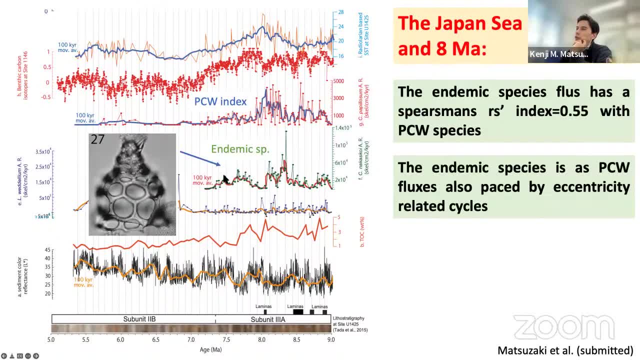 we check if how both curve species are correlated. We only have a Spearman's index of 0.55, so it means that, yes, the endemic species is partly related to the inflow of the PCW, which is related to the PMOC and low eccentricity. However, 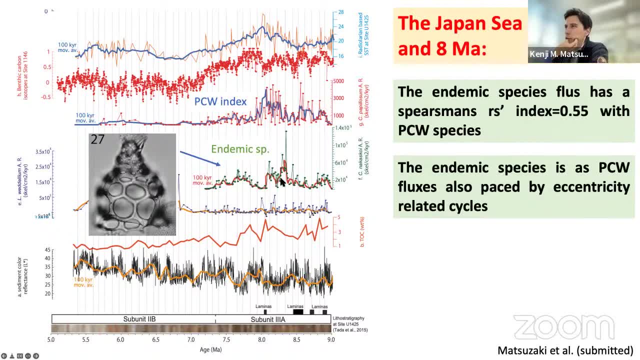 you should have other mechanisms for allowing it to bloom, And because we do not have many strong evidence for that, but because at that time the winter monsoon was weak, so we suggest that the summer monsoon was pretty strong. So as a speculation, we propose: 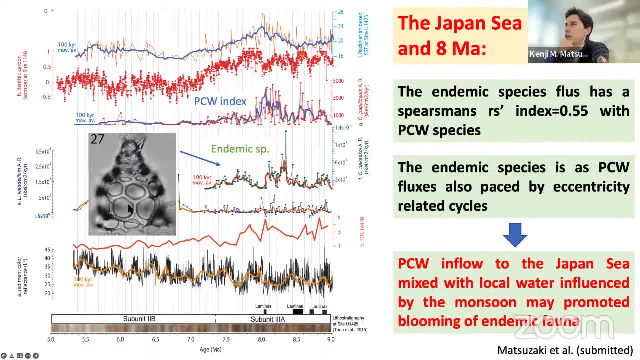 that the occurrence of this endemic species is related to both PCW inflow due to strong PMOC and probably to local water influence by the summer monsoon And probably the end of the whitening of the summer monsoon around here is one of the 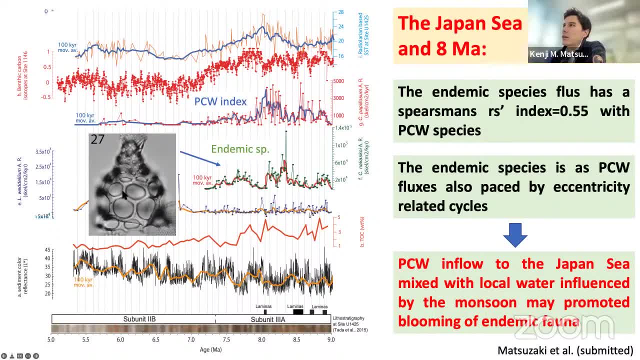 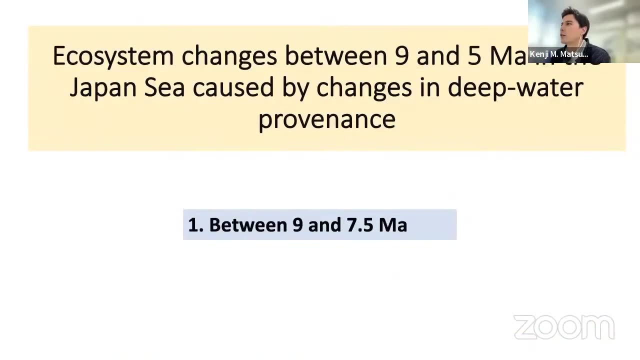 factors causing this species extinction. but the monsoon is not likely the main factor causing the decreasing inflow of the PCW water into Japan Sea and this is the reason we want to discuss now in our second part. So from 7.5. 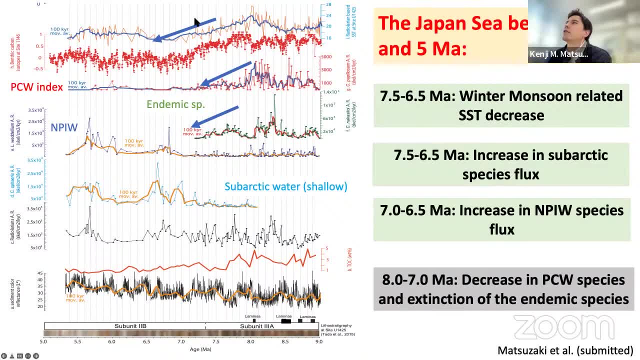 million years. you have a decreasing sea surface temperature, decreasing PCW species inflow and the extinction of the endemic monsoon. Instead, you have an increasing flux of NPRW species and increasing fluxes of species which infer migration of the subarctic water. 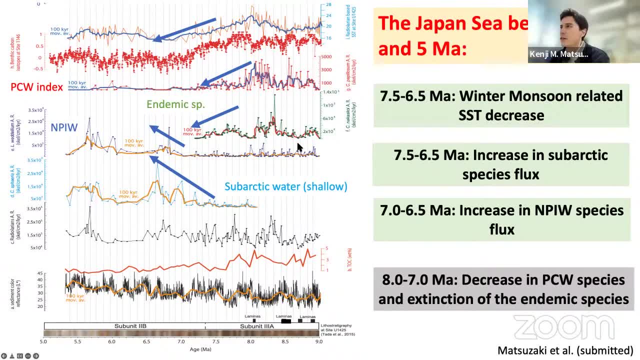 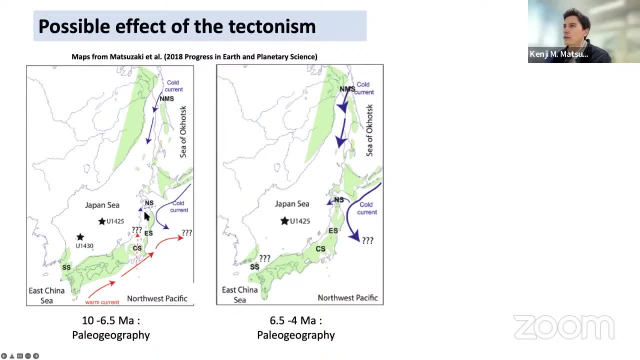 So how to explain this factor? So the first, we have to consider the tectonics, because, as I show you here, you know, here you have a, our solid site is here, and from 10 to 7.5, and from 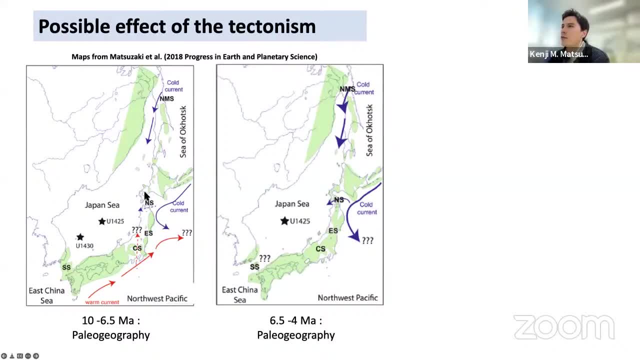 6.5 to 4,. you have an uplift of the east part of Japan, which cause we have more land, and also you have a showing of the strait about here, and previous studies suggested that this strait actually showed from about. 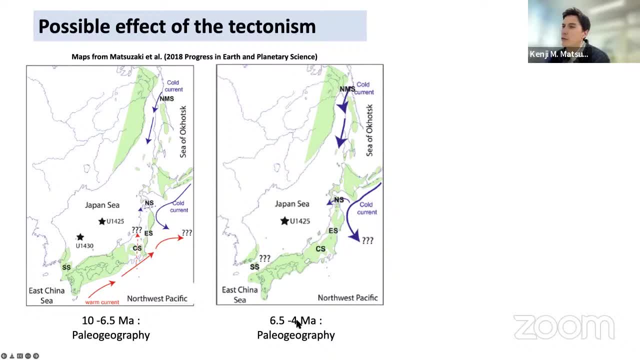 1,000 meters to 500 meters at 4, between 10 to 4 million years. so it's progressive. it's not. it cannot occur rapidly, but progressively. you have a showing of this strait from 1,000 meters, about 10. 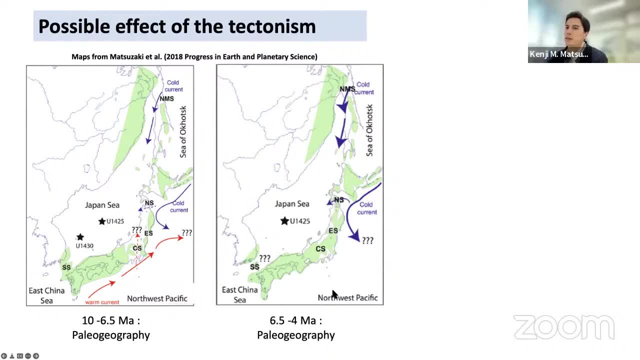 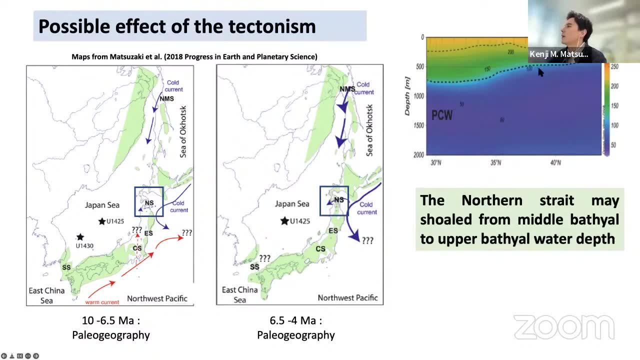 million years to 500 meters, about 4 million years. so we suggest that the tectonics should be of importance because, as you can see, the PCW here well, it's up to the area. so here it's about. 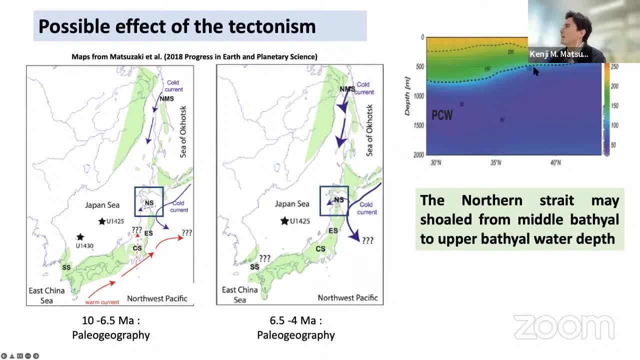 the latitude is about 35 to 40, so if, for example, if the seal depth gets shallow from 1,000, from 1,000 to 500, it will automatically prevent PCW inflow. so as a possibility, we suggest that the tectonics 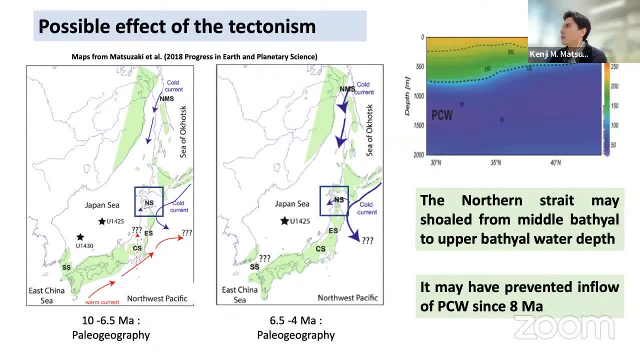 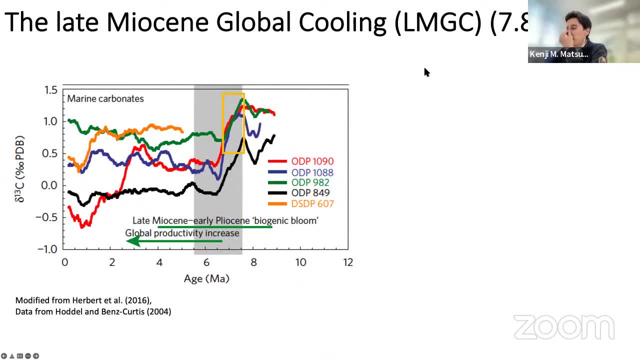 may be one factor which stops PCW inflow to the Japan Sea, But there is also another important factor. it's here, here, as you can see, it's here. it's the carbon isotope curve from the Southern Ocean, compiled in Harvard 2016,. 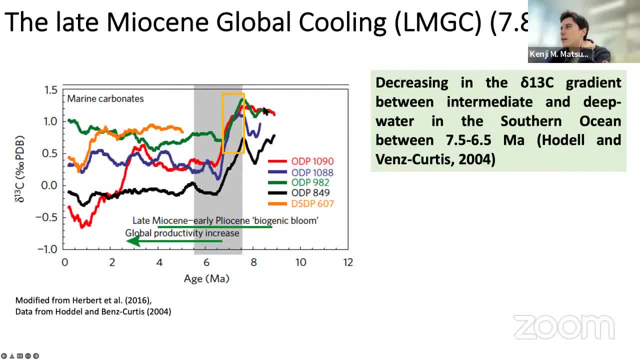 so I think here it's. I do not remember which is what, but the red, green and blue indicate carbon isotope from the intermediate and deep water of the Southern Ocean, and the important thing is that from 7.5 to 6.5 million years. 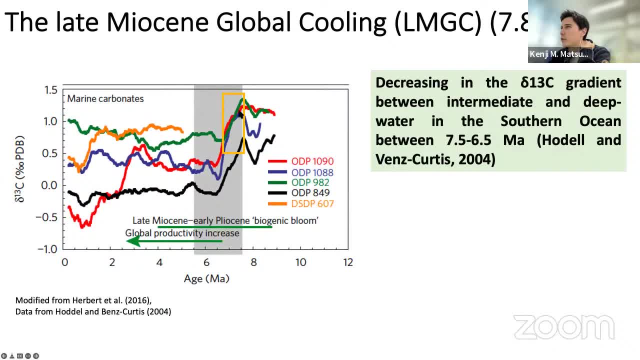 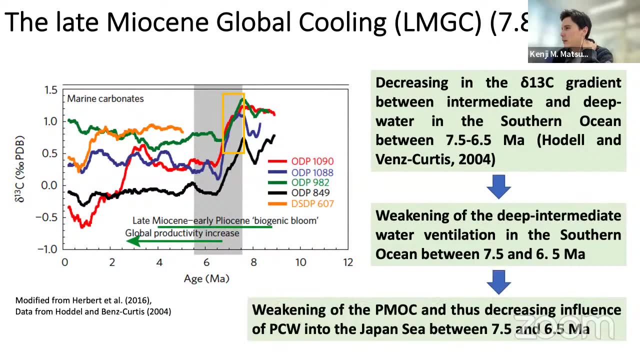 there is almost no gradient between the shallow, between the intermediate and deep water in the carbon isotope signal in the Southern Ocean, which was associated to a decrease in ventilation, a weakening in the ventilation of the Southern Ocean, which will in fact cause a weakening. 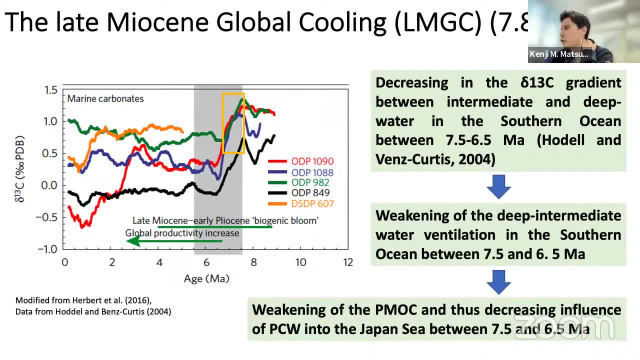 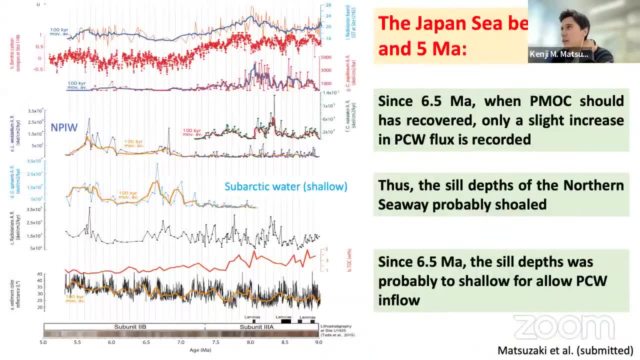 of PMOC and if PMOC is weakened automatically, you will have a lower production rate of PCW, and the Japan Sea may have been sensitive also to this event And actually this weakening of the PMOC might occur between 7.5. 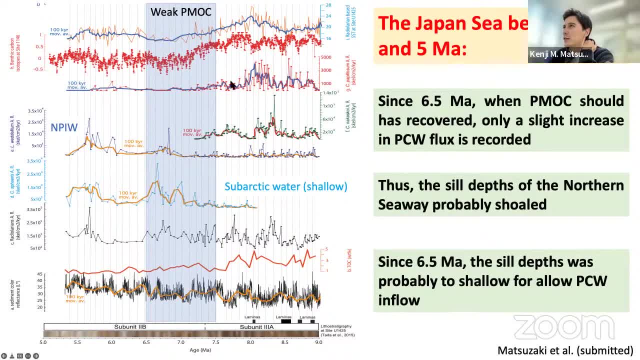 and 6.5 million years, which is over there. So, as you can see here, it is 500 kilo years after the first decrease in PCW species here. but so this part is likely related to tectonic, but for this. 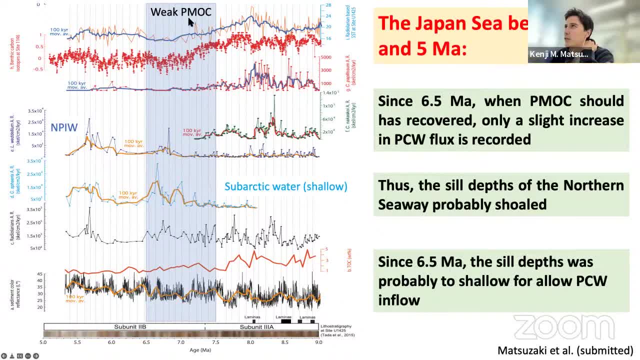 to this part, where you go almost to zero. it is likely that the PMOC weakening was the last event causing that the Japan Sea was not influenced anymore by PCW. And for support of this hypothesis, after 6.5 million years, 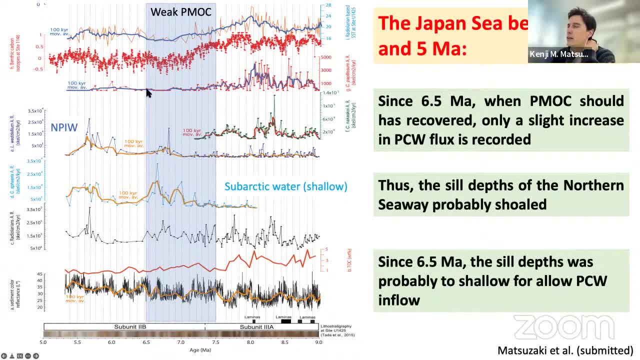 when you have a recovery in the ventilation of the Southern Ocean deep water ventilation. there is no big change here, So it means that from here to here, the Northern Strait of the Japan Sea continued to shoal and it was probably too shallow. 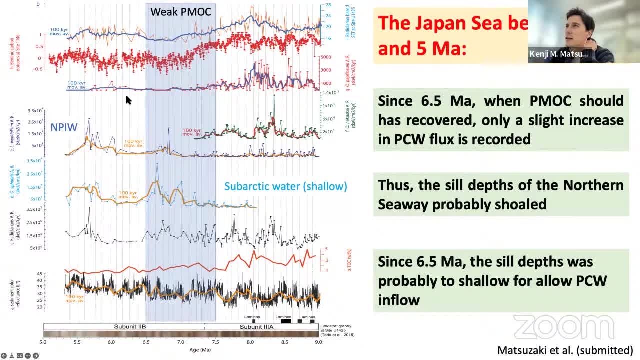 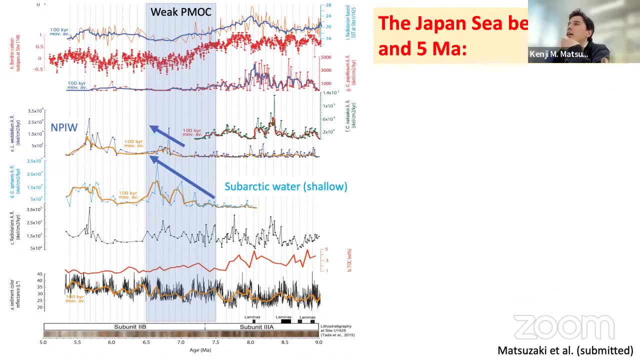 Once it was recovered from the weak PMOC. it is likely that, because of tectonic, the Northern Strait was too shallow to allow high PCW influx, like before. So this is how we interpret this result And for this data. well, it was. 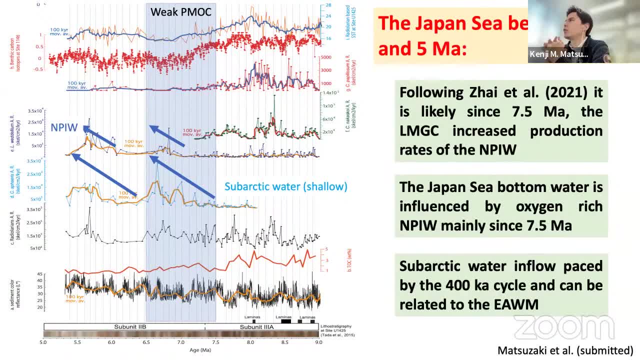 already discussed many times and it's not so new, but we just say that we are in a close agreement with SAI 2021, and it is likely that during the LNGC there is an increased production rate in the NPNW water. 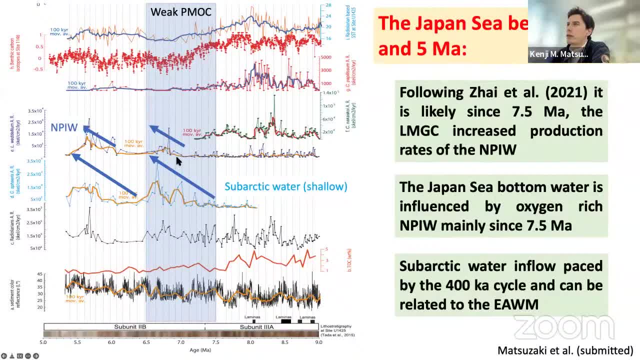 which became the unique and dominant deep water influencing the bottom water of the Japan Sea, And it was probably related to the increase to the inflow of the sorbatic water which, as you can see, high peak, occur every 200 or 400 kilo years. 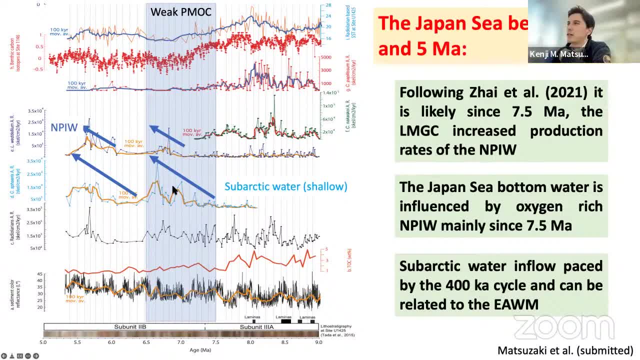 which can be associated with a winter monsoon signal. So we propose that strong winter monsoon causes a thousand shifts of sorbatic front in the Japan Sea And, on the other hand, in the North Pacific. because of the global cooling, you have an increased production. 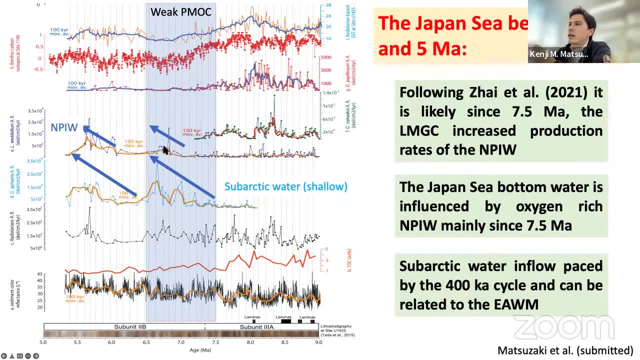 rate of the North Pacific intermediate water and the Japan Sea likely more shifts from a temperate subtopic summer monsoon climate oceanography to a more sorbatic climate oceanography around 6.5 and 7.5 million years. So now I just wish to. 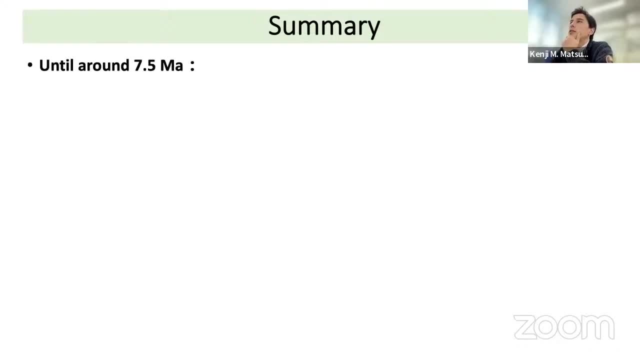 summarize this part. So until 7.5 million years. we propose eccentricity-based PMOC, allow inflow of Pacific central water into the Japan Sea and it is more probable that a mixing of PCW water with local water influenced by the summer monsoon. 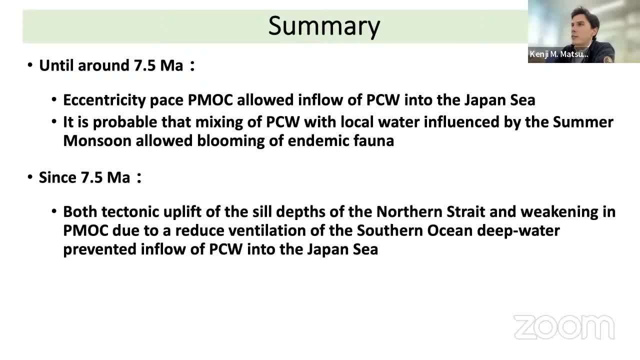 allows a blooming of endemic fauna And since 7.5 million years, it is likely that both tectonic of the seal depth of the Northern Strait and a weakening in the PMOC due to a reduced ventilation in the Southern Ocean prevented PCW inflow into the Japan Sea. 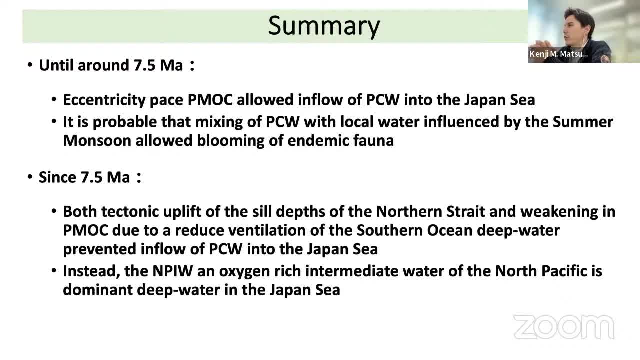 Instead, the NPIW, which is an oxygen-rich intermediate water of the North Pacific, became the dominant deepwater influencing the Japan Sea, And the winter monsoon may allow a blooming of NPIW, but I forget to discuss this point. 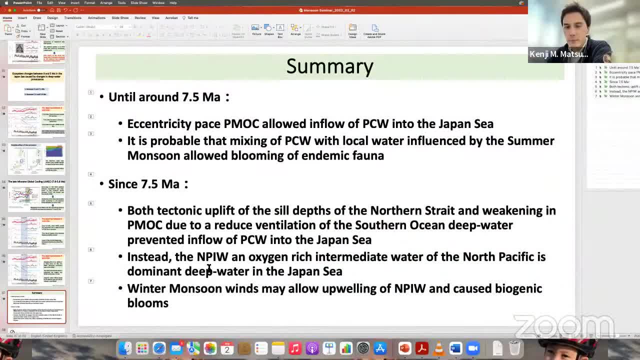 That's all I have for today. Thank you, Great Thank you. So let's see There we go. Okay, So please remember to type in any questions that you have in the chat For our speaker today. I do have a question for you. 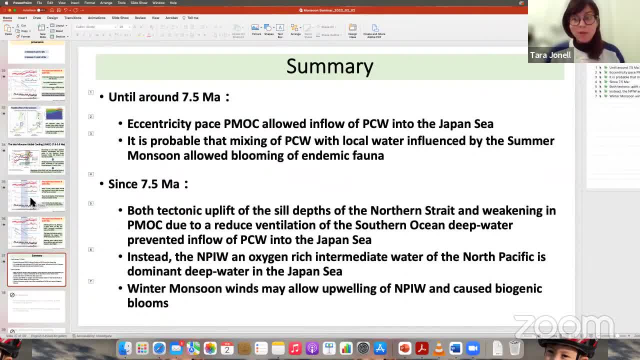 as everyone's gathering their thoughts. So you have some great data in terms of the temperature and the ventilation in the Japan Sea, kind of, I think, on a local scale, with the geographic distribution of some of your species as well as kind of broadly. 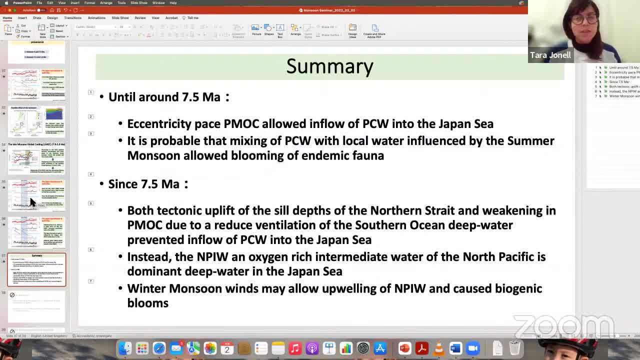 So do you have any evidence for salinity from any of your radio learning? Do you have any evidence for salinity from any of your marine species, either locally, with increased winter monsoon discharge or with, maybe, changes within the Sea of Japan For the shallow water? 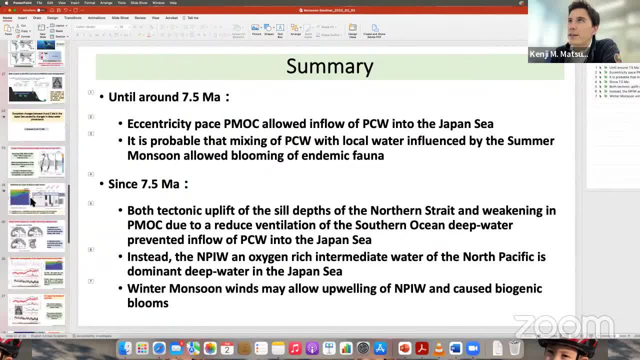 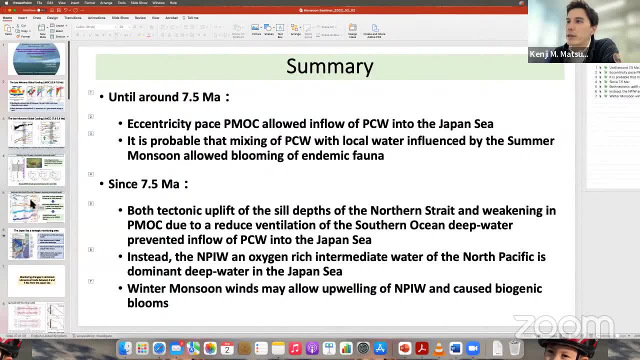 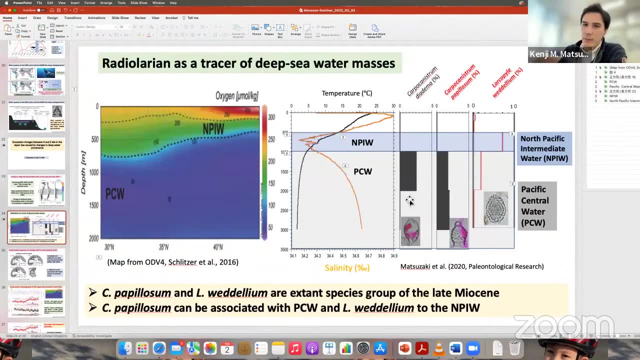 you're speaking? yeah, Yeah, probably shallow water. Yeah, yeah, But again I understand I did not plot it here, so I will go to the slide. I have this type of data with other. here I mainly focus with the deep water, but 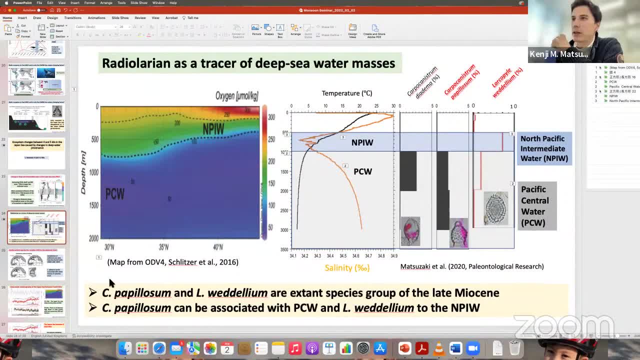 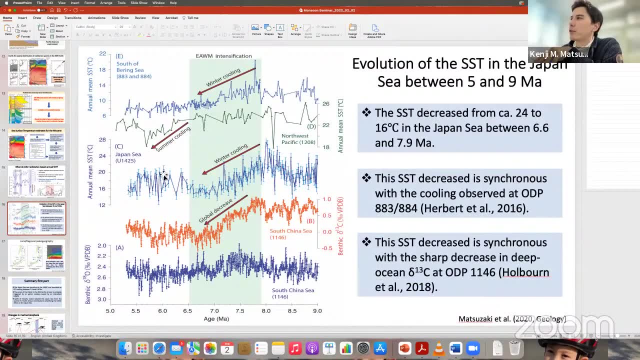 but, yes, how to say that? Well, I do not have the data in this PowerPoint, but, for example, when you can see in this SST profile, when you have for this period, when you have relatively high sea surface temperature, you have high flux of. 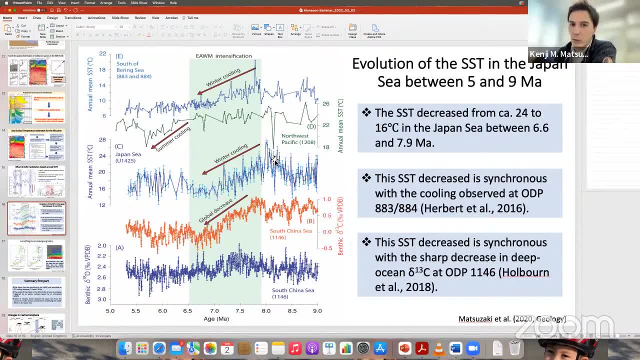 species tolerant to low salinity and warm water, Ah, cool. But they are not related to Yes, yes, yes, Cool, great, Yeah, just because the fact that you have such an intensification with such a change in temperature. I think it would be. 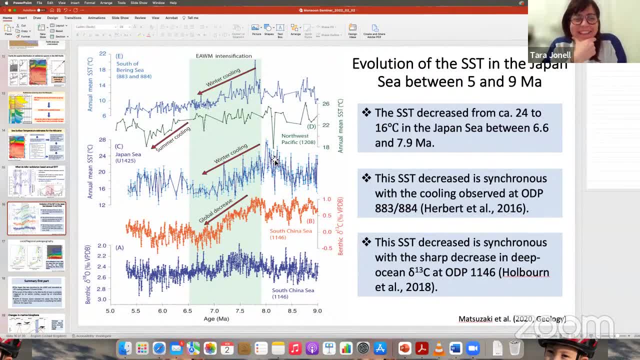 just the. I mean there's a lot going on. Yeah, it's a lot of great data. Actually, this could be associated with also an increase in salinity, because from about here, you have, you do not have or you do not have. 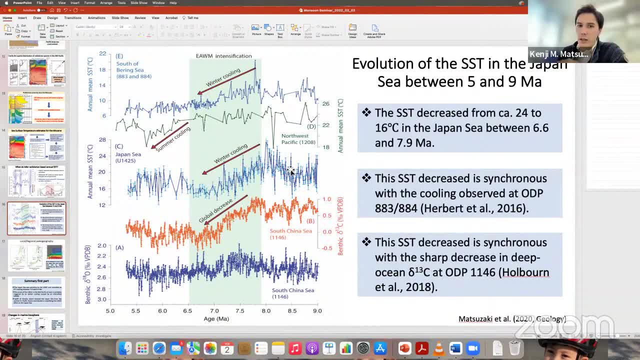 species with high temperature and low salinity tolerant species. You shift from fauna at this boundary. Ah, cool, okay, So it's also consistent with the winter monsoon intensification. I think Nice, great, thank you. Oh, I see that. 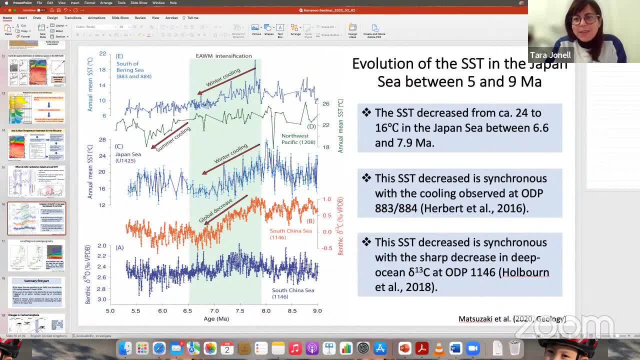 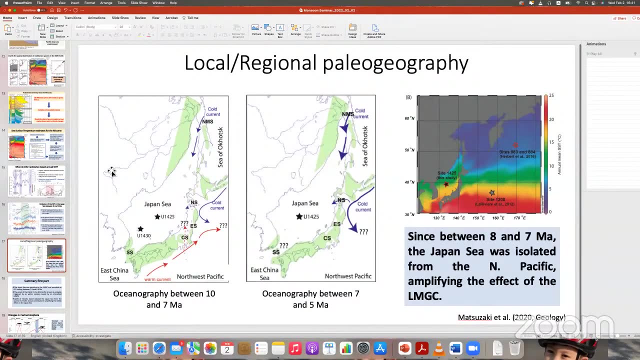 Anne has her hand raised. Anne, would you like to ask your question? Yes, good morning. Thank you very much for this really interesting talk. I'm very curious about this North Pacific influx of water masses. I think it's very exciting because we know. 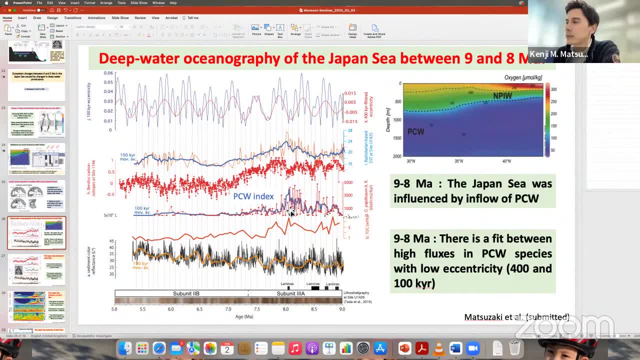 so little about the North Pacific circulation in the Miocene? And in terms of the radiolarians, what would be the why? would you have a specific assemblage of radiolarians associated with this water mass from the North Pacific? Sorry, I'm not sure. 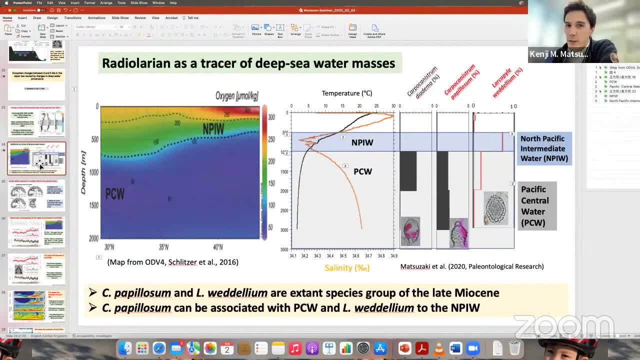 why I have. are you speaking about this graph, This figure? Yeah, I'm curious about why you would have a specific assemblage of radiolarians. Are you speaking about ecology? Yes, yes, Okay, thank you very much. 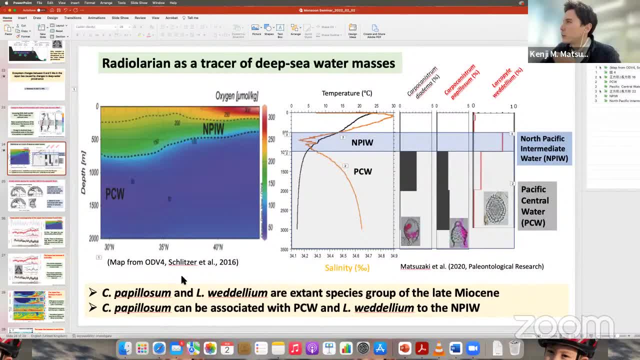 So it's a very complicated question. Sorry, Here it's just observation. you know, I looked at the plankton samples and of course when you look at the plankton you have very high diversity in the upper areas with many, many species, and when you go down, 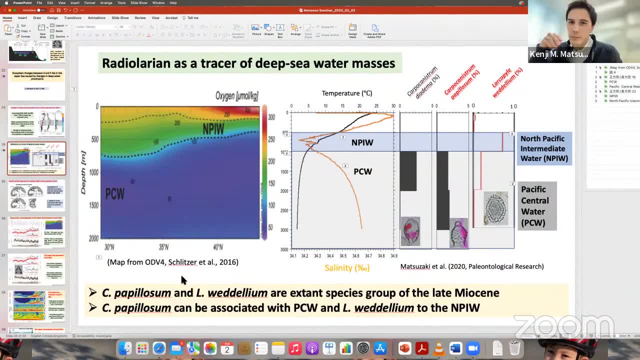 you get automatically very few species diversity And these species, today at least, prefer these water depths so which, as you can see, is very salty, very oxygen-poor. so, as a hypothesis, it might be that they may have shifted to the deep in water depth because of the 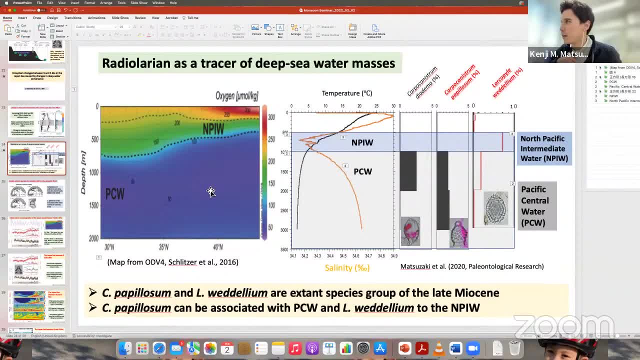 hyper-competitivity in nutrients in the shallow water. Did I answer you? Yes? yes, I think it's more related to migration due to competition for get food normally, Thank you, But if you just look at the data, it can be. 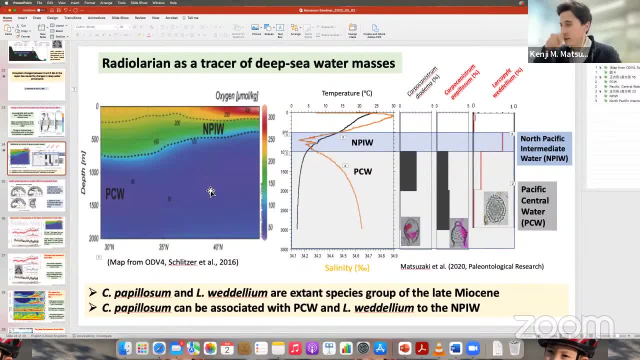 seen. yeah, yeah, it can be used for trace of this water mass at this time And the most interesting thing is that if you go in the lower latitude, when you get more sustained influence of the inter-servatic water, these species abundance in the surface sediment. 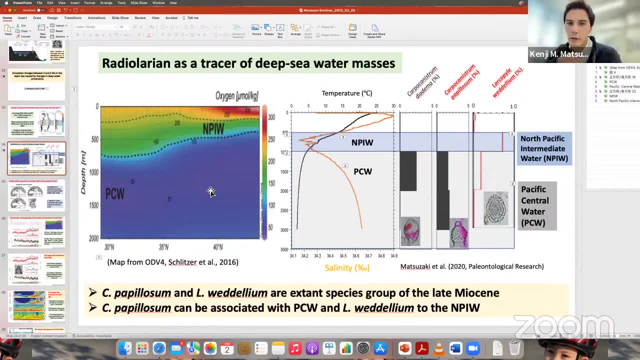 is higher than when you go in the high latitude. So I think that it's quite suitable proxy for try to monitor these water depths, these water masses. I'm sorry, Okay, Great, Thank you very much. Yeah, thank you, We have a. 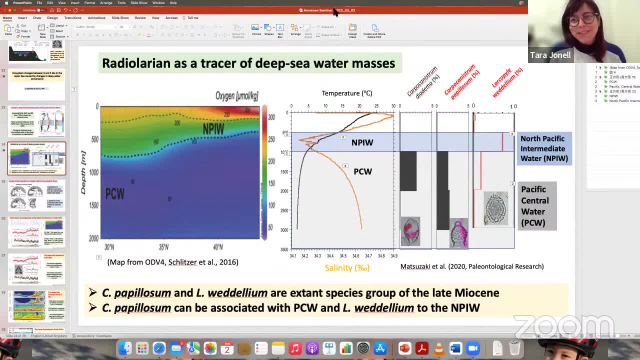 couple of comments in the chat. Really, Yeah From Mark and Antje. Thank you, Complimenting Thank you, yeah, And then. so just if anybody has any other questions, please come in or raise your hand in Zoom. 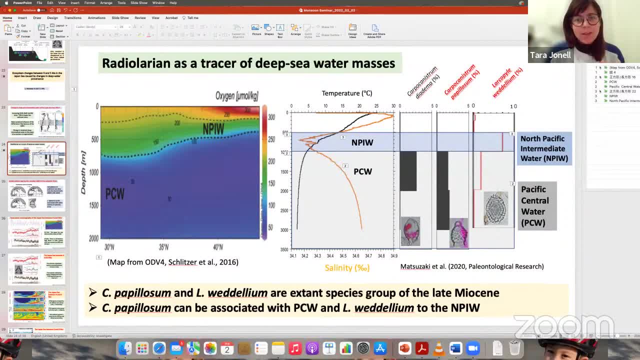 So I had another question: Considering the amount of data that you have, were you able to establish any type of biodiversity metric at all, or is that kind of beyond the scope Biodiversity? well, of course, yes, we, because if you count each species, 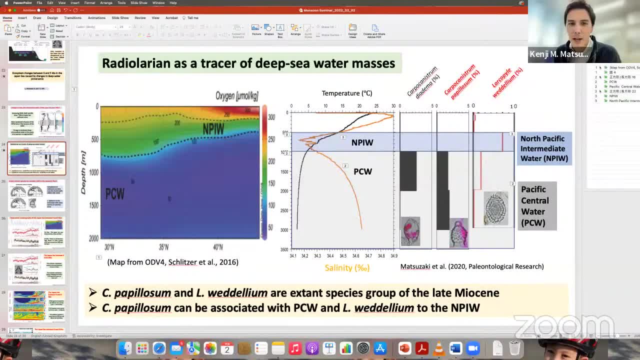 it's possible to provide such type of data. yeah, However, I did not. I'm sorry. Okay, there's only so much we can talk about. It's possible, but yeah, Great, We'll give everyone a moment if they have any other questions. 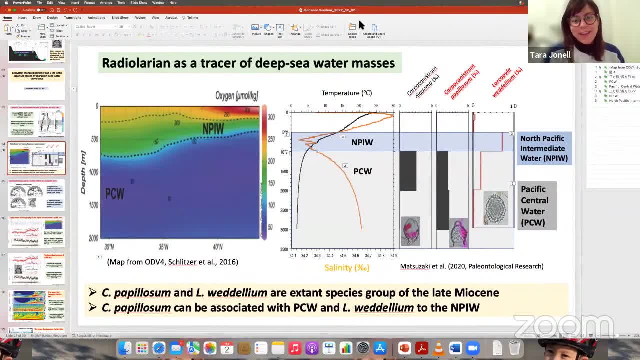 Okay. Well, thank you so much for your talk today, Kenji. You have a wonderful talk Again, great excellent data. We'll just see what's coming out of your lab. And so, before everybody runs away, oh wait, there's. 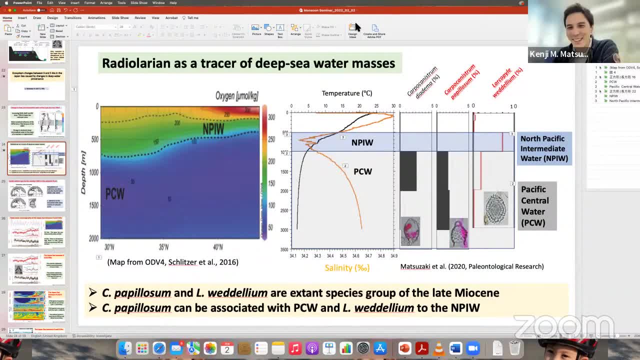 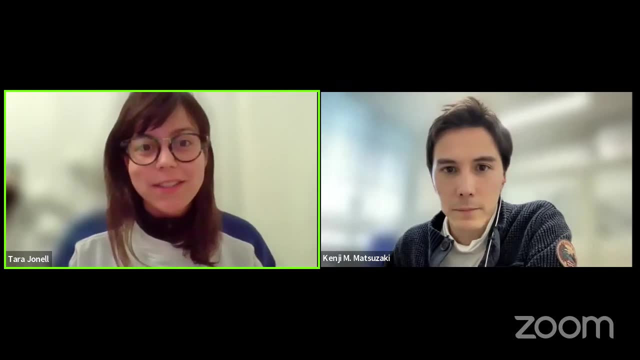 wait, that's applause hands, not applause hands. So, before everybody runs away, please remember to attend the talk that is next week, on the 9th of February, for Mahyar Matadi, And with that I hope everyone has a great rest of your. 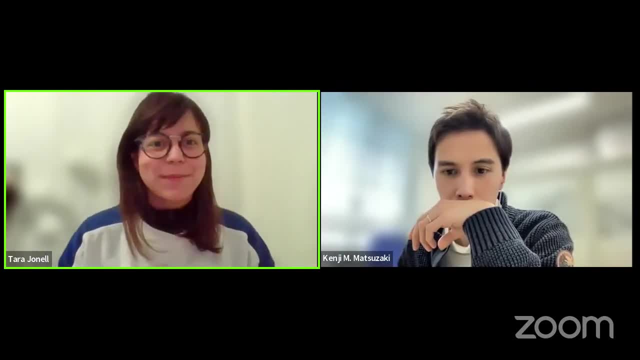 day And again. put your hands together for the speaker. Thank you All right, Thank you, Bye everyone.